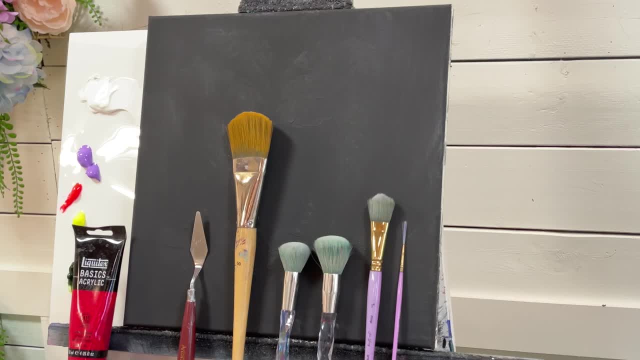 going to show you how to use it. I'm going to show you how to use it. I'm going to show you how to use it. And this brush set is released for the third time this April 2024.. So I'll have a link below where 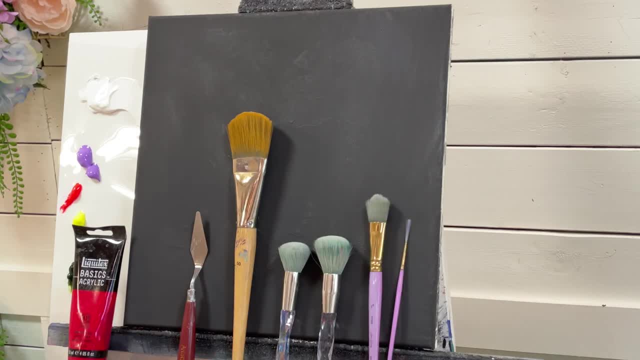 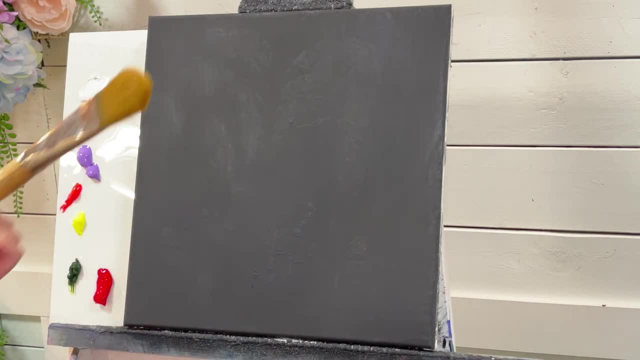 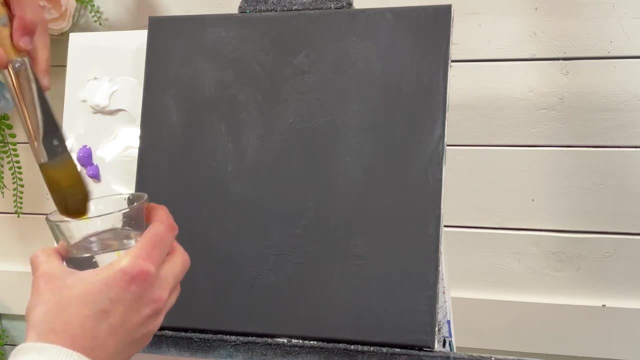 you can go. click on that. It will take you there. Thanks everyone, I'm going to squeeze out my Napsol Crimson Now. what we need to do to begin this painting is take a large brush. Here I have my fifty and I'm going to be taking a little bit of water and I'm just going to wet down. 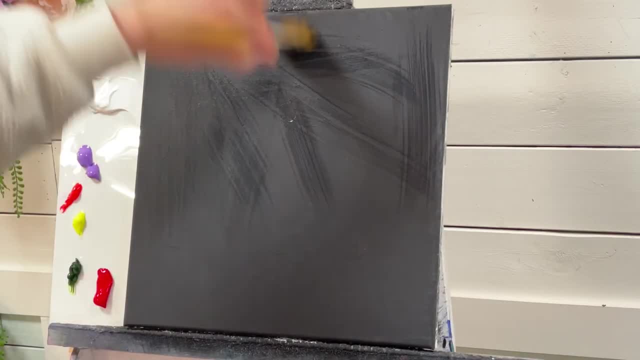 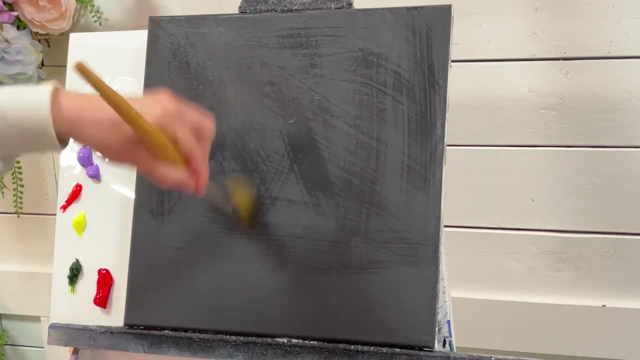 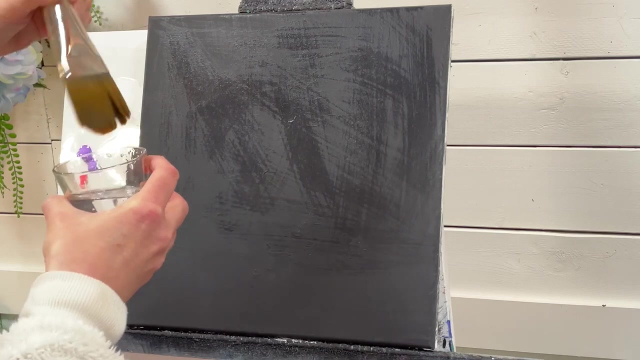 the canvas a little bit. This will help the canvas take the paint better and help me get a nice soft airbrushed blending effect. I'll probably still need to add a little bit of water during this process. However, I'm going to just take a little bit more on the end of my brush, like this: 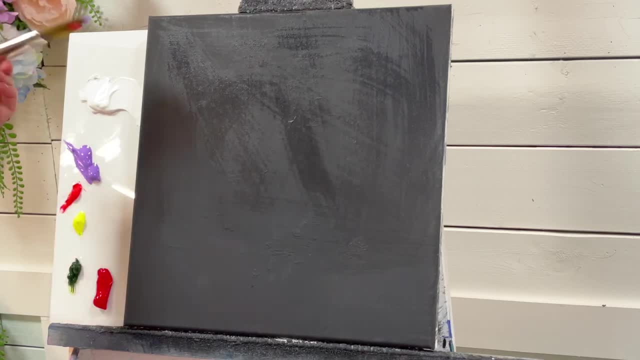 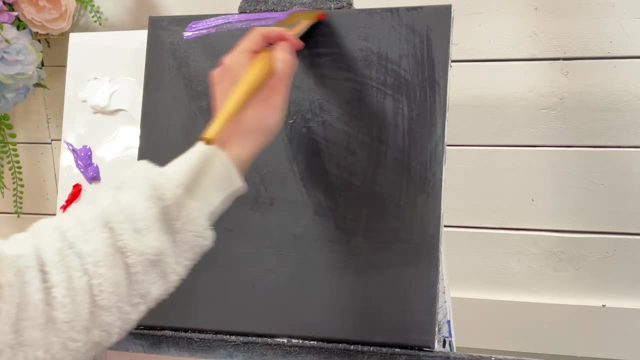 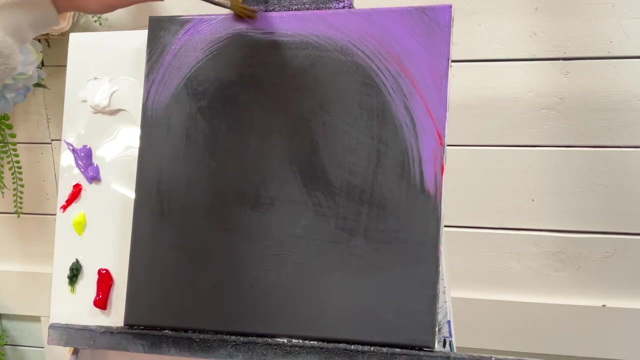 and I'm going to start off with purple and I'm going to add: I accidentally picked up a little bit of red. that's okay, because we are going to be using red next. What I'm going to do is come around the edges with the purple and we're going to gradiate into our red yellow. 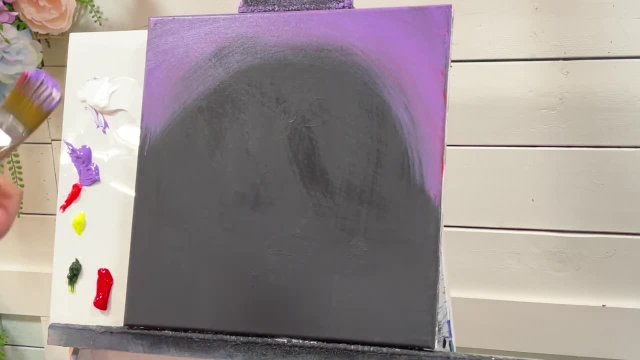 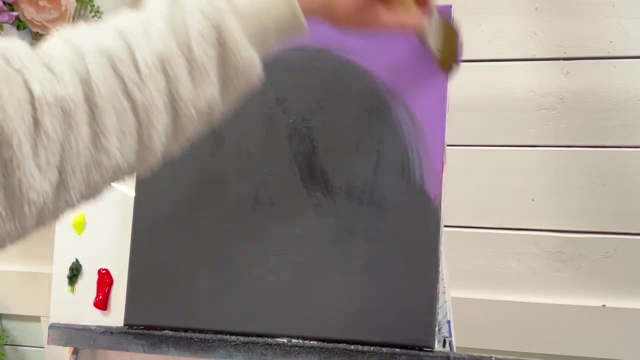 Now, as we do this, I'm going to pick up a little bit of white, because we're painting on a dark canvas. I'm going to add a little bit of white just so that it stays a little bit on the brighter side, Otherwise it's going to dry to a 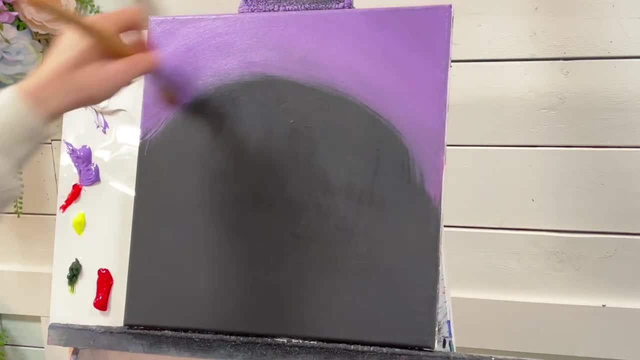 fair amount of white, I'm going to add a little bit of purple. I do want to paint on a black canvas, though for this, because we're going to get the most depth this way and it's really fun to see how you can create that working on a dark canvas. 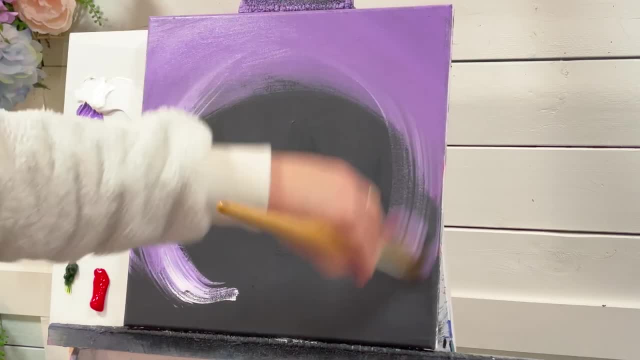 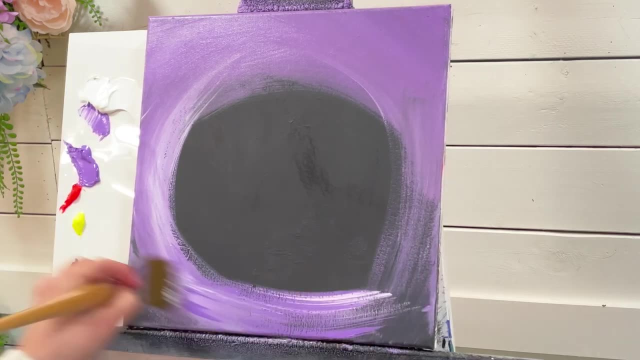 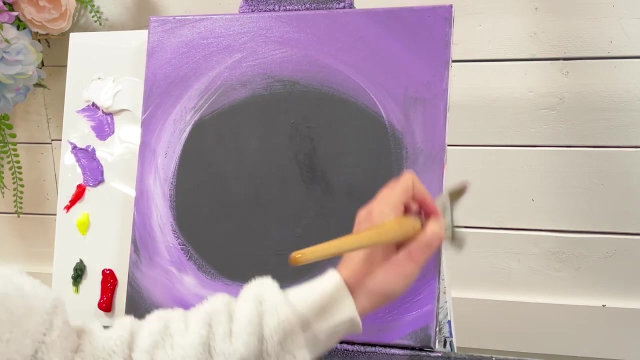 So I'm just going to go around, Even though we're going to cover up part of this down here, I just want to go around and add this, because there's going to be little hints of this purple in between the green and our flowers and it's going to look really pretty. 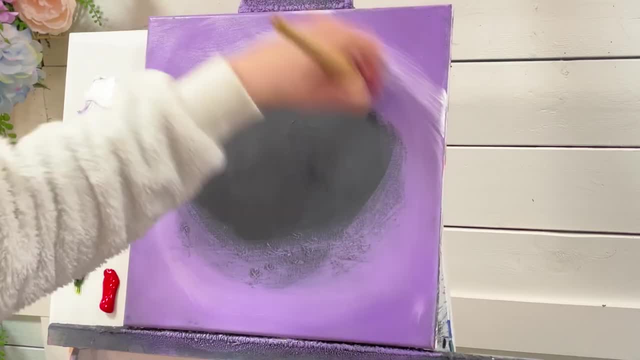 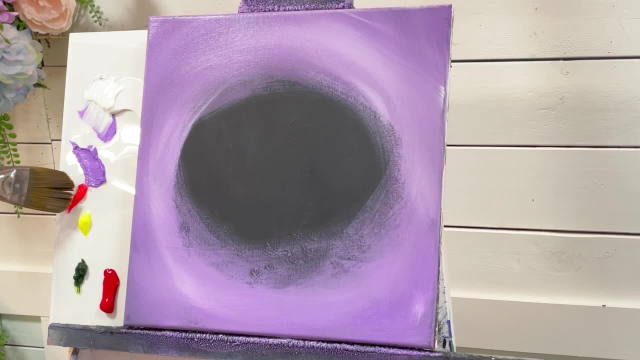 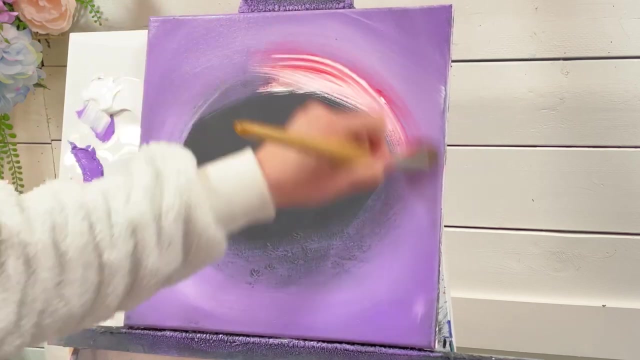 I'm going to take a little bit of white again, some more white, go over this some more. And I'm going to take some red and white now and I'm going to apply this partially over the purple, So we're going to get a little blending in there. 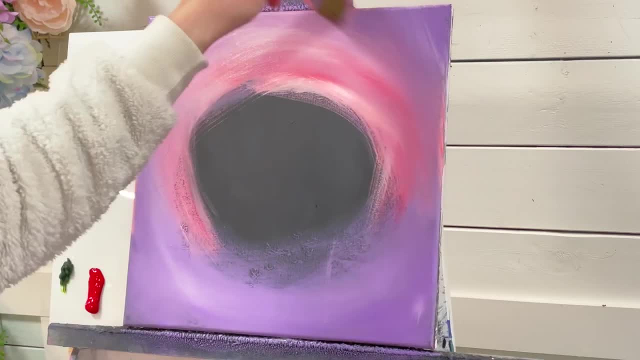 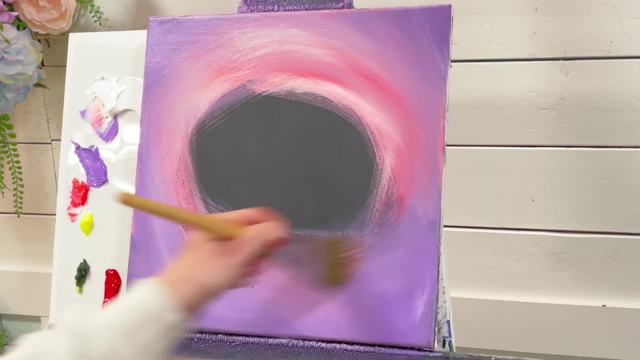 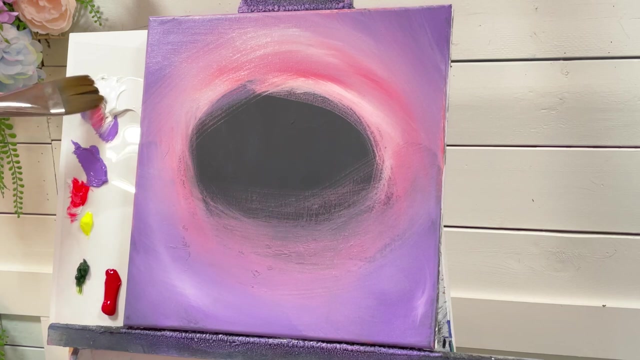 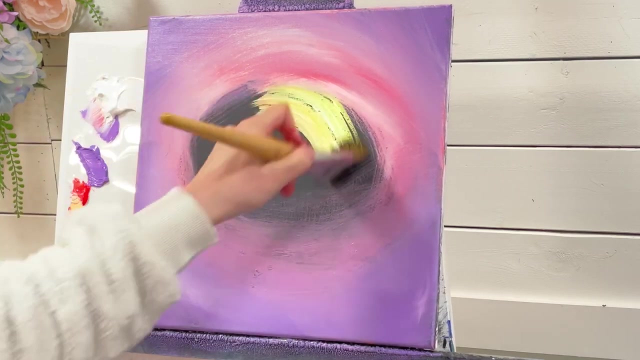 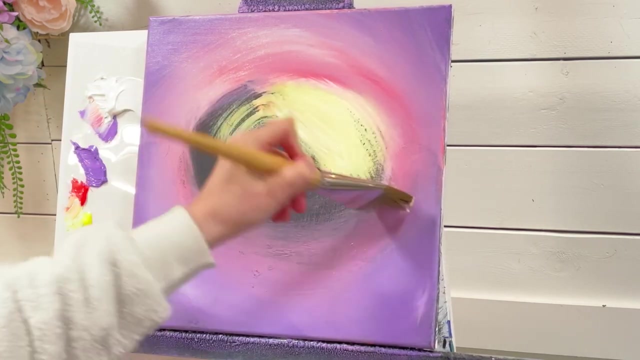 So see how pretty that is, mixed with the purple. and now I'm going to take some white and some yellow, a little hint of that red, and I'm going to start right about here. it's important to have a little bit of white in there, otherwise the yellow is going to dry green. so 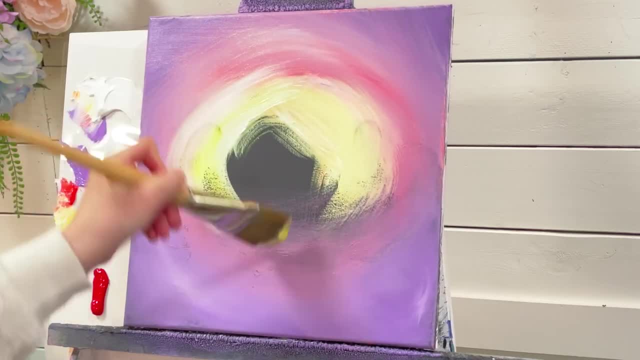 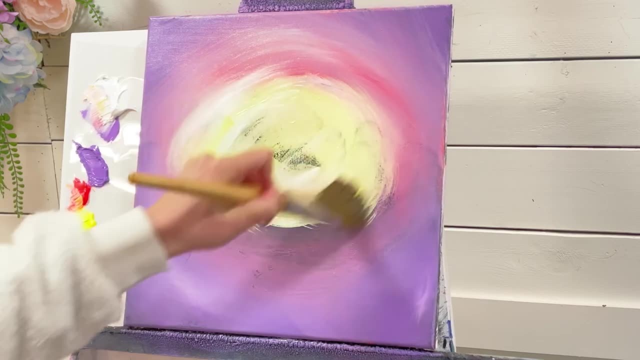 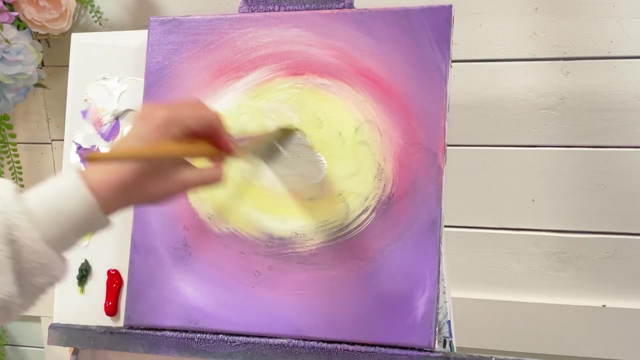 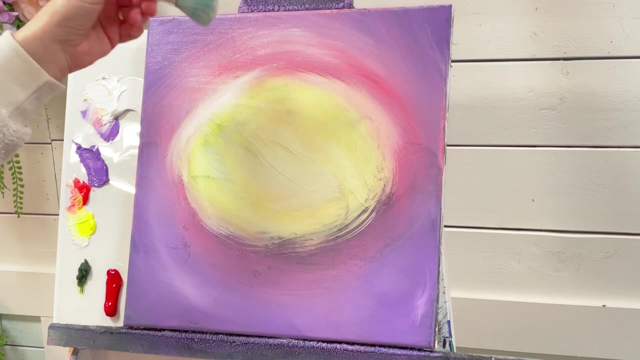 we're going to blend that into our red. I'm going to add a little bit more white in the center. this is where our dry mop brushes come in handy. you want to do this technique, apply this technique to wet paint. so I'm just going to soften by going around in. 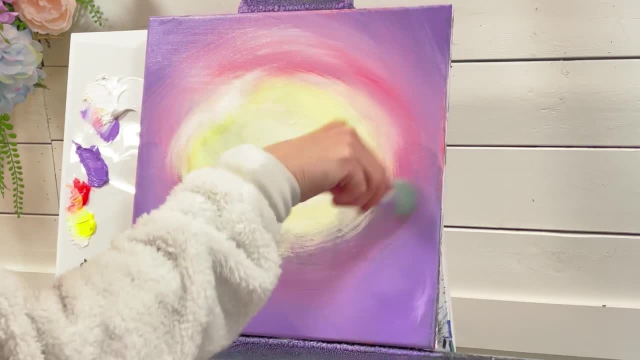 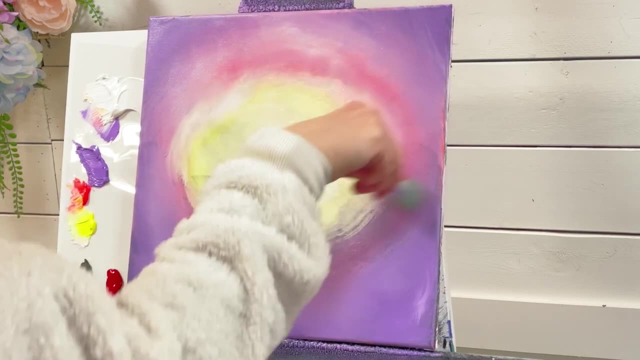 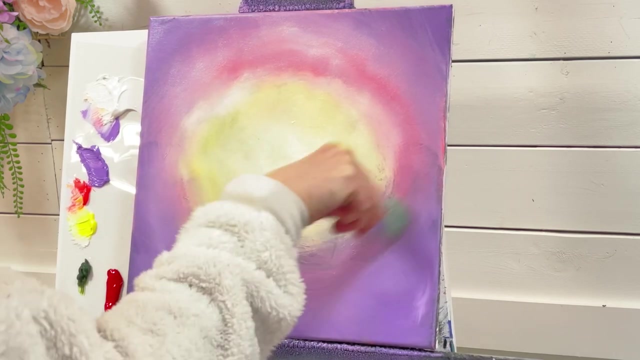 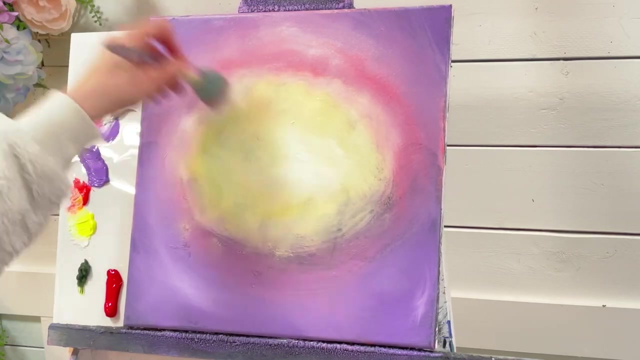 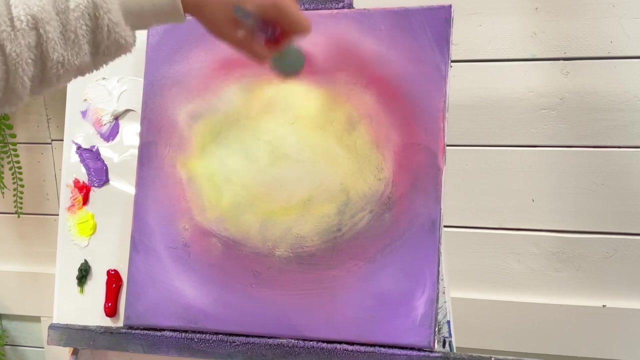 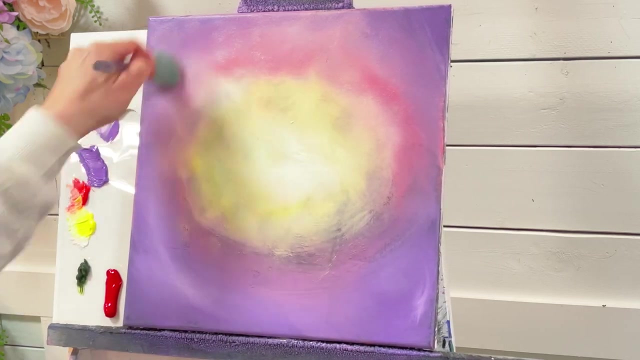 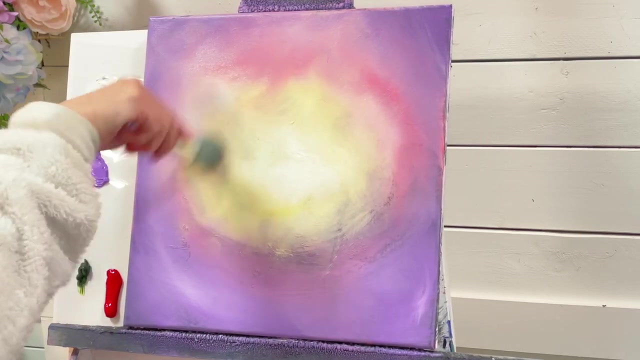 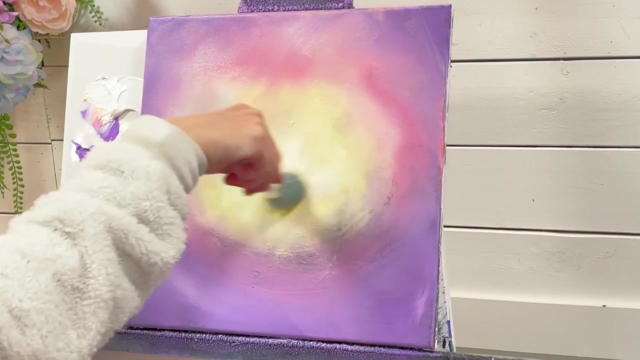 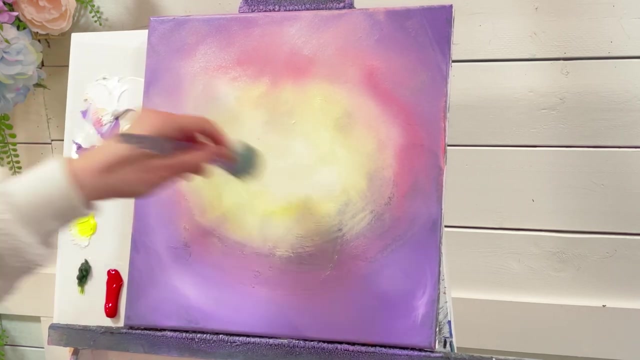 little circles now. you don't need- you shouldn't need- to push very hard. you can lightly pull as well and bring some of that yellow start in here. just continue to go around in little circles and bringing it out to the purple. okay, the next thing I'm going to do is rinse that brush out and I'm going to go. 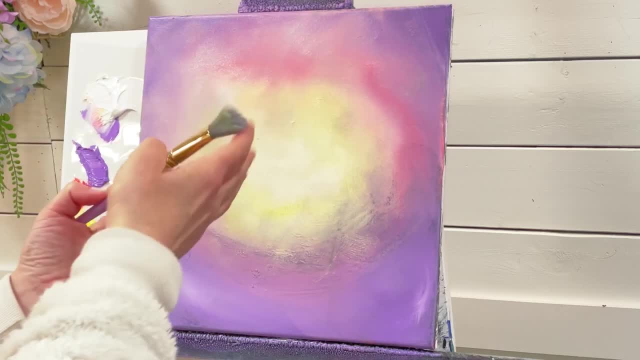 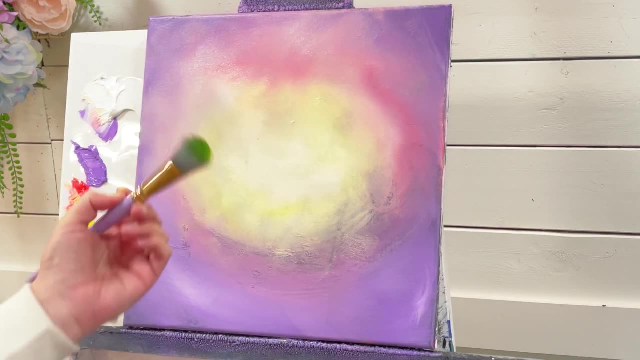 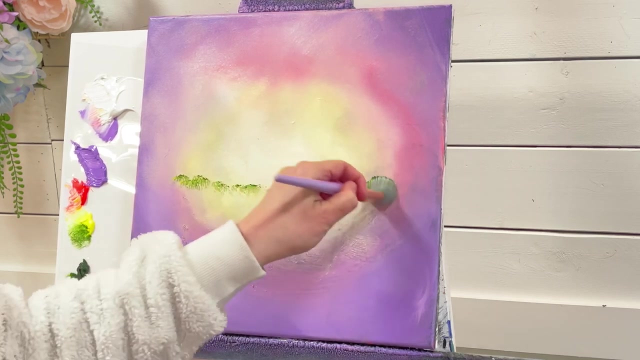 over to my smaller mop brush and I'm going to take my brush and I'm just going take a little bit of green, a little bit of yellow and I'm just going to start pushing and tapping along here for the beginning stages of our flower field. 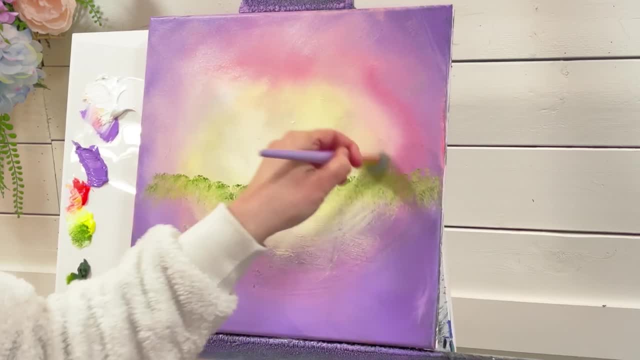 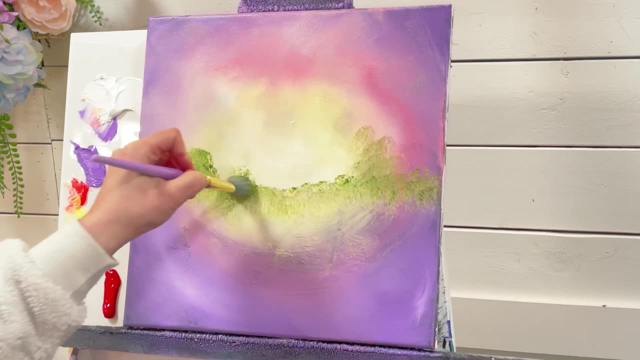 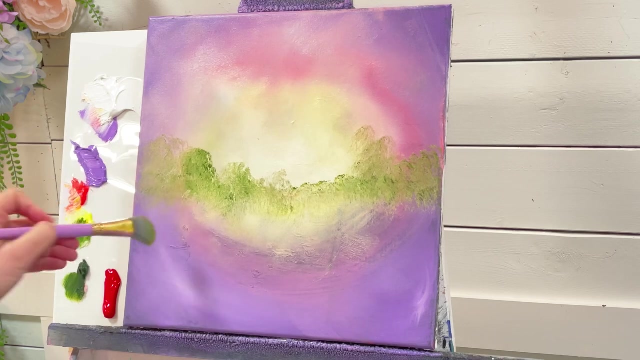 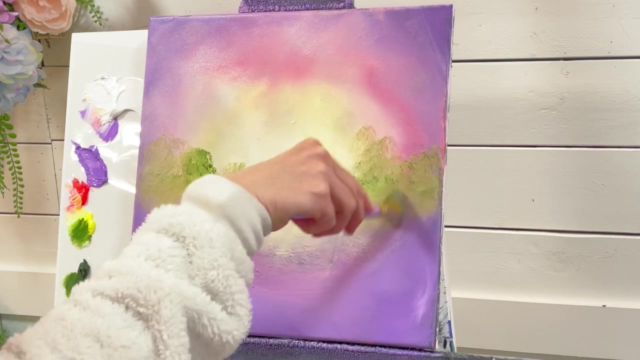 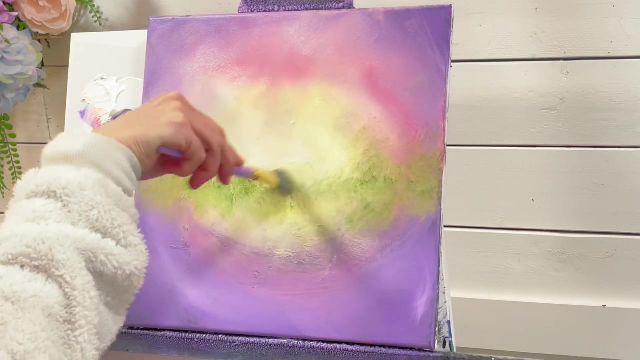 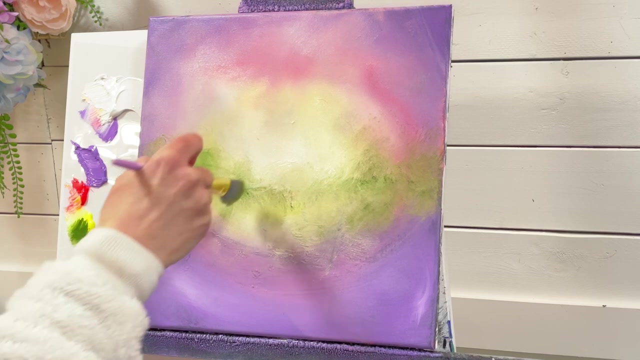 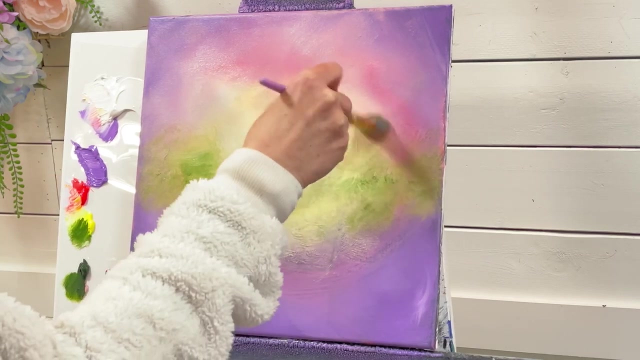 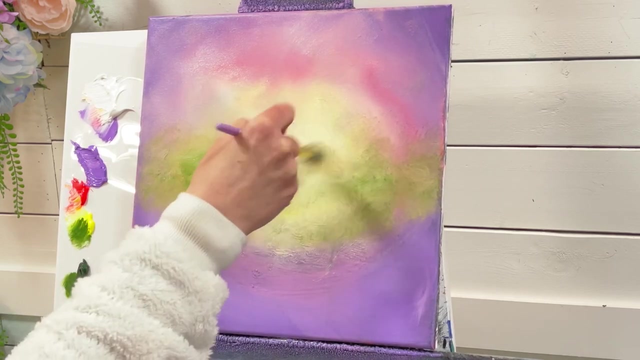 Some grass, some bushes, Tap and dab that around, bring up a few little higher tree areas, And then you'll just go around in little circles blurring that up and softening. Okay. Okay, I'm going to take a little bit more green. 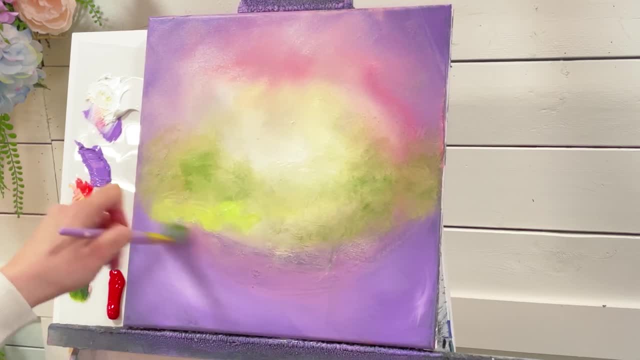 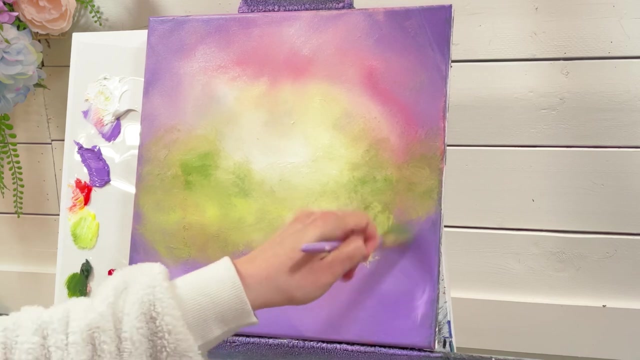 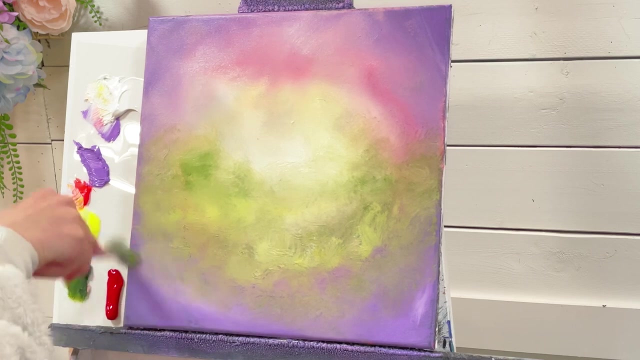 I'm going to take a little bit of green and yellow And then I'm going to rub it in a little bit. Okay, Okay, Okay, Okay, Okay, keep layering. I'm going to take more of the green this time. 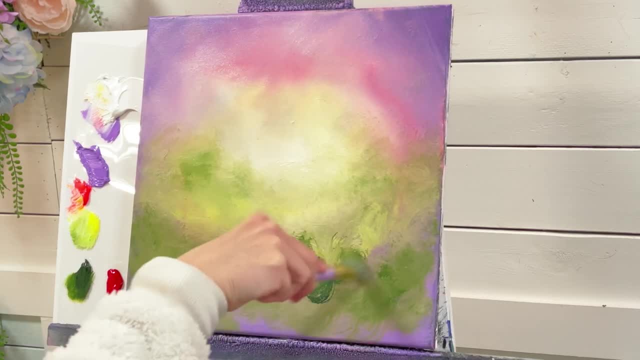 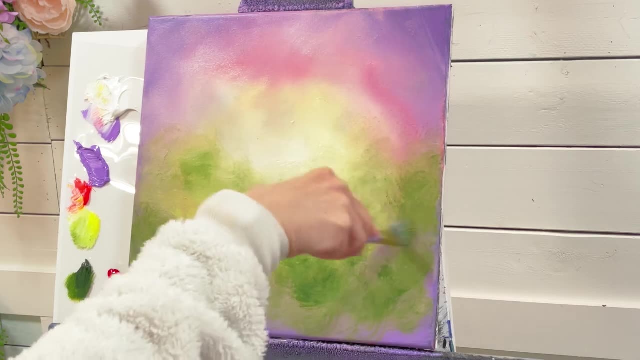 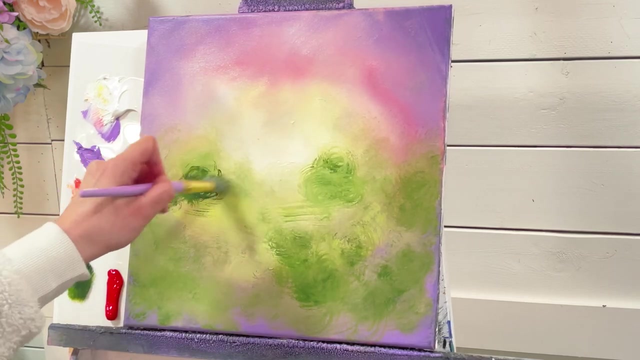 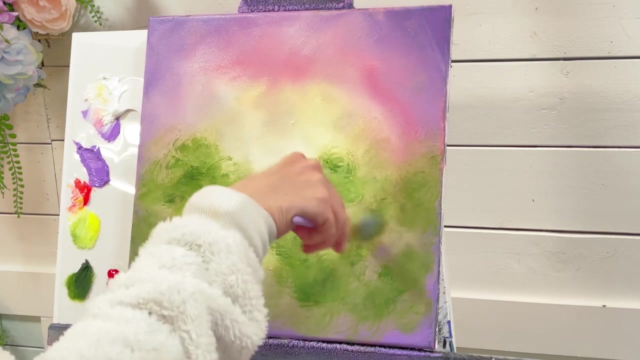 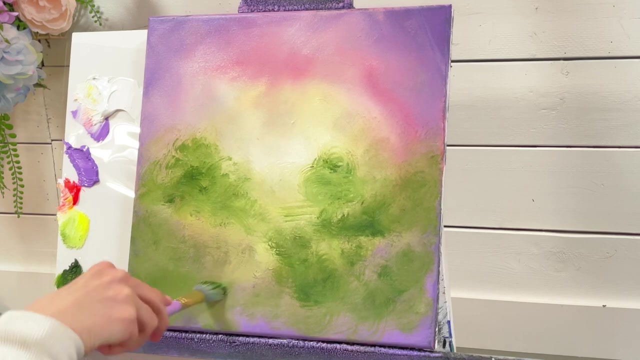 I'm going to start to layer a little bit more. The paint is going to start to dry a little bit now and we'll be able to add some darker areas like this. Okay, Okay, Let's take our dry and clean mop brush. 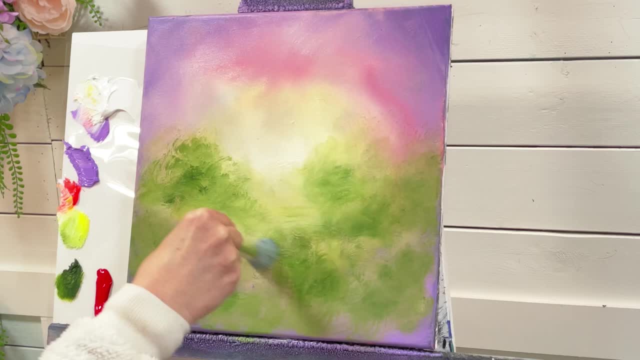 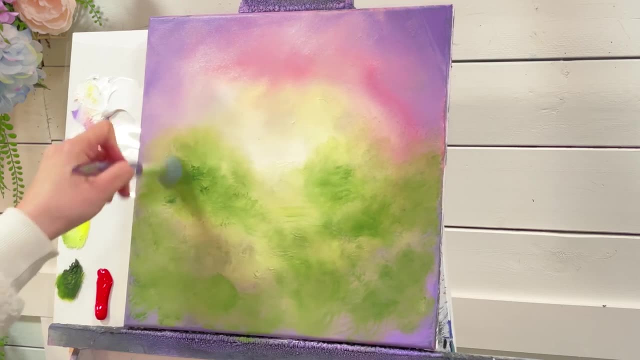 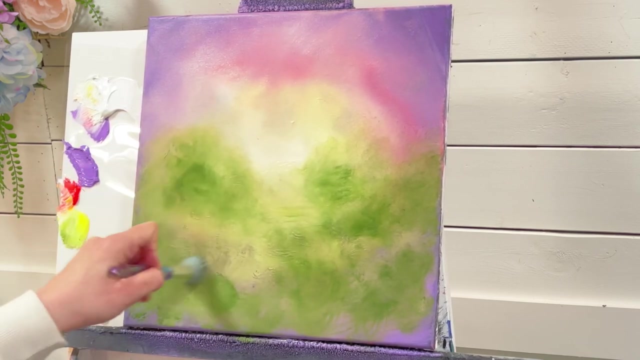 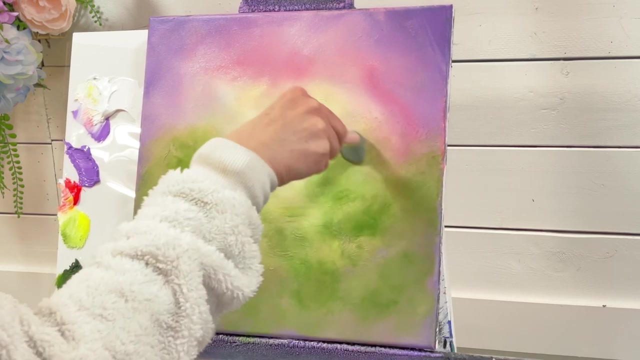 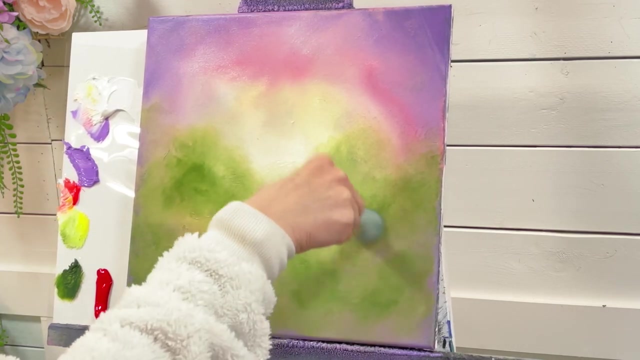 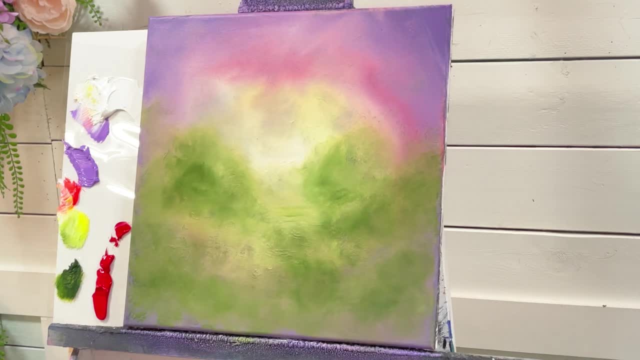 And what I'm going to do is I'm going to take my palette and I'm going to apply it on the is. add a little bit more yellow. I'm going to get a little fresh area here of yellow, just so that it's I'm not dipping into a little bit of green that I made with that yellow I'm going to use. 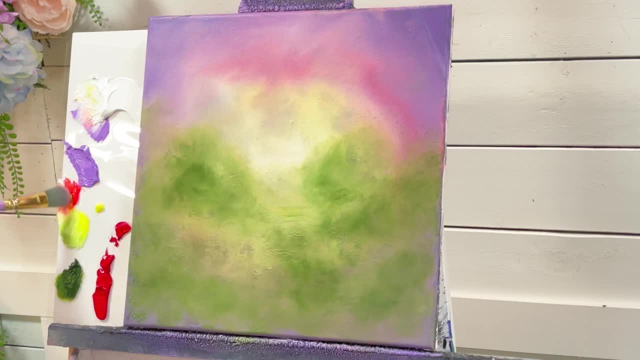 another mop brush and I'm going to take a little bit of red, a little bit of yellow and a little bit of white and I'm just going to go around in this area here in a soft circle, take a little bit more push and twist, push and twist. 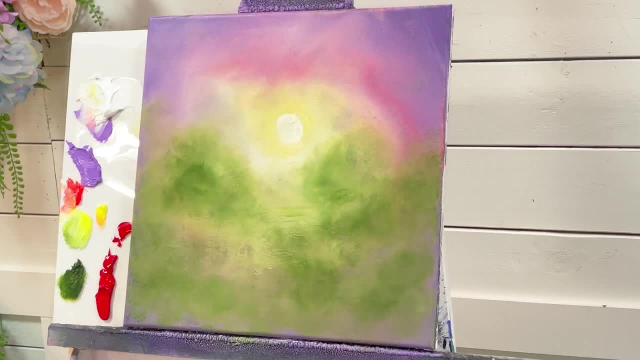 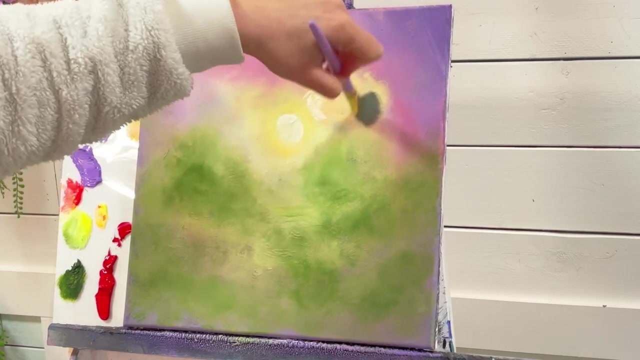 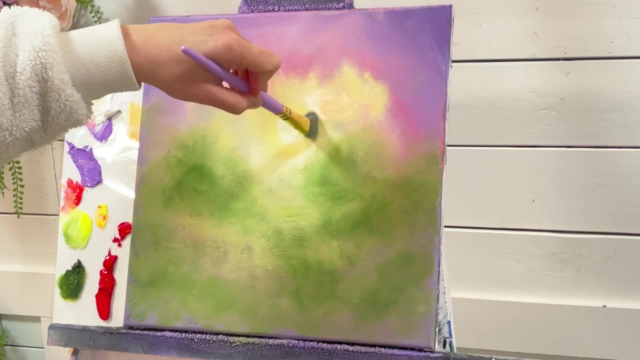 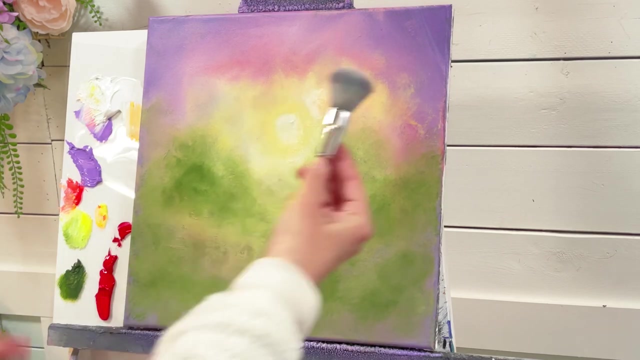 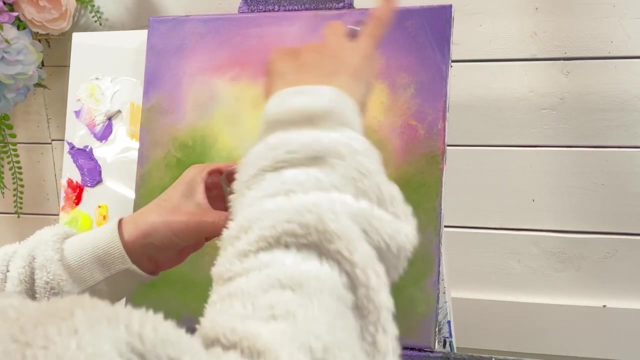 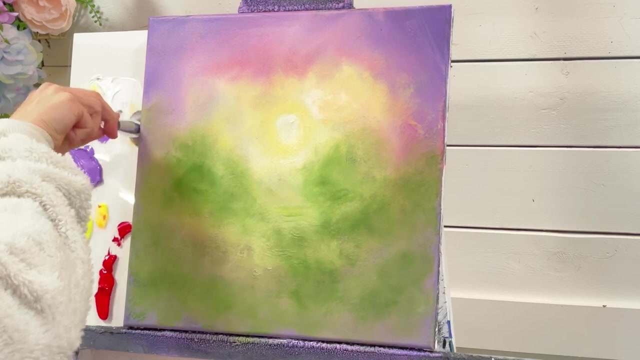 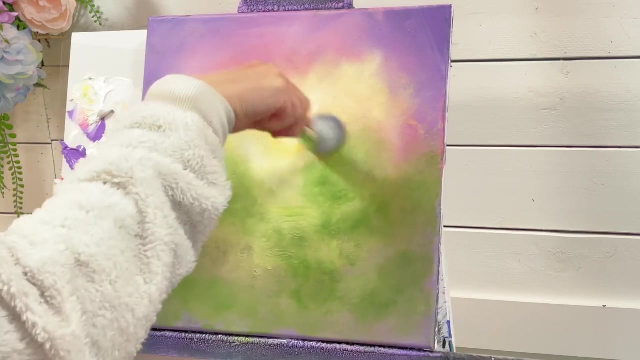 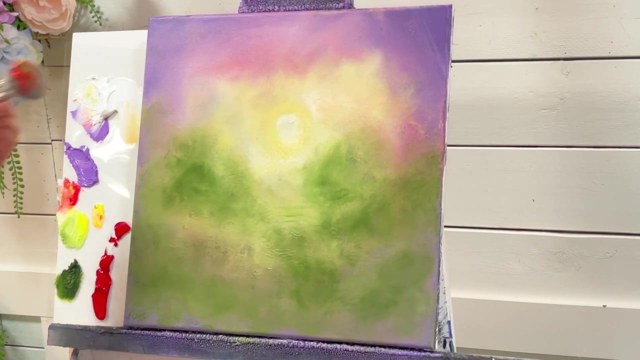 take a little bit more yellow and red, get really close to the white. add a tiny bit of water to your brush, if you need to. I'm going to go over to one that's a little bit larger. Add a little bit of water- you don't need a lot- and just soften a little bit more. 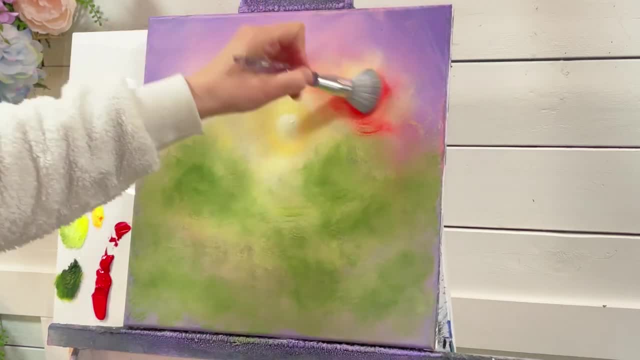 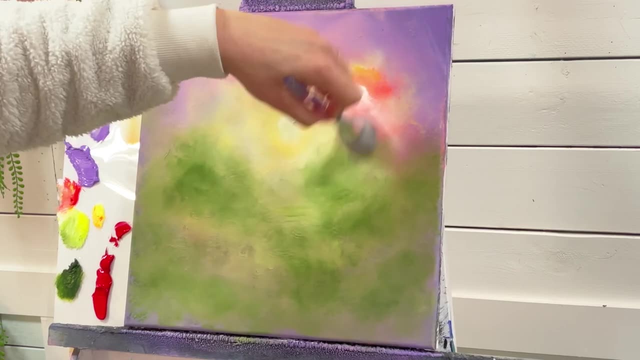 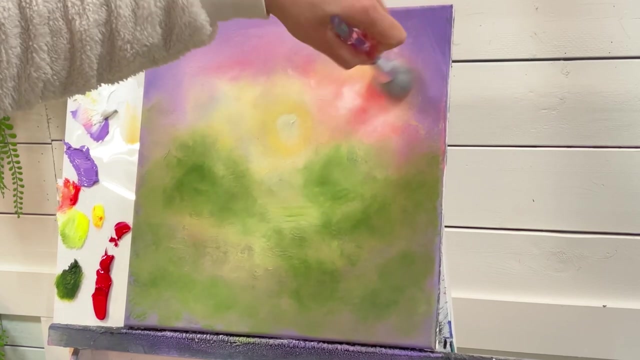 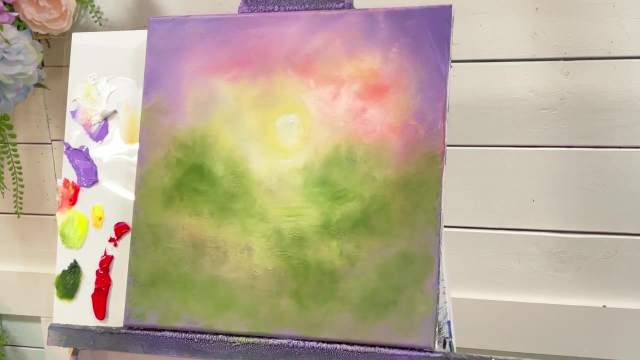 red, a little bit more yellow and a little bit more white. Look at that beautiful shade of pink that we make. You've got to remember to soften it after. Okay, then I'm just gonna dab my finger in some white. I'm gonna place it right there in the middle. Now I'm gonna come in with my 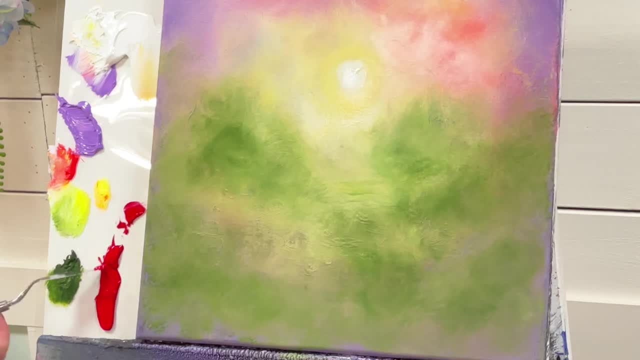 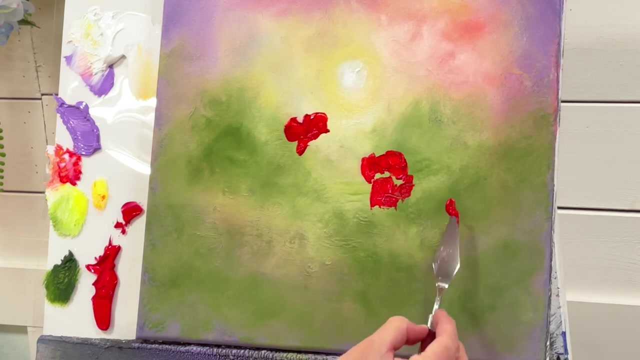 palette knife. I'm gonna take both of my reds and I'm just gonna start pushing and tapping. The paint is going to be quite thick when we do this. Now, if you want these to be red poppies, they can be red poppies. It could be any. 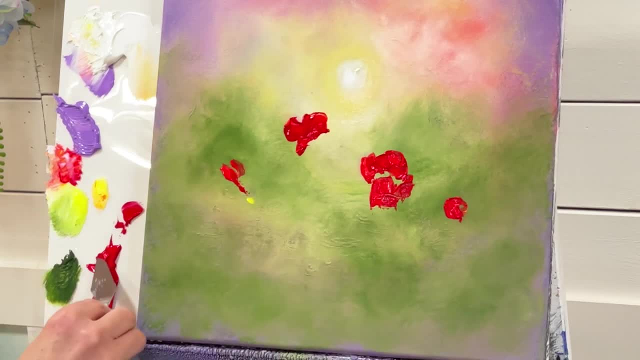 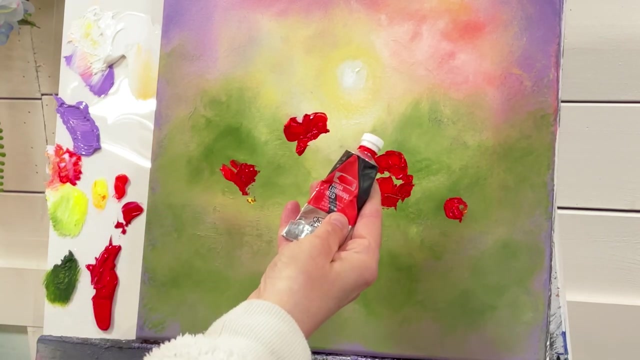 flower that you want, and you can use a different color if you want. I love red, though like red just really stands out. Now I'm going to apply some more ofize my Luminous Red, the design line: You just dab a little on there. 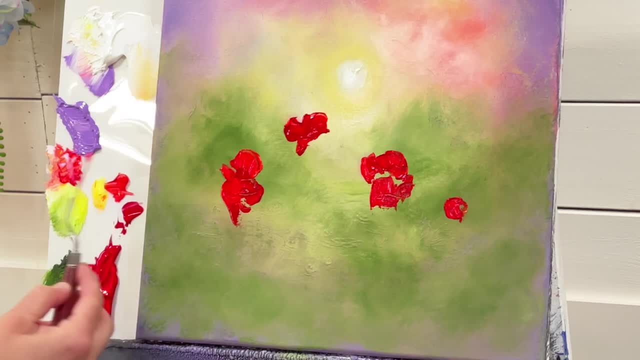 Push around gently with your brush or pushف. I knew I was going to do that. I rarely use a palette knife, so I'm probably going to call this a brush a few times. So the bright neon red that we're adding is going to give us a little bit of a well, they're luminous paints and it's going to make the petals look luminous and light filtering. 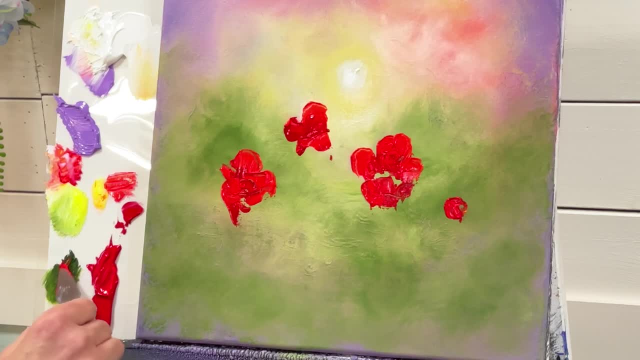 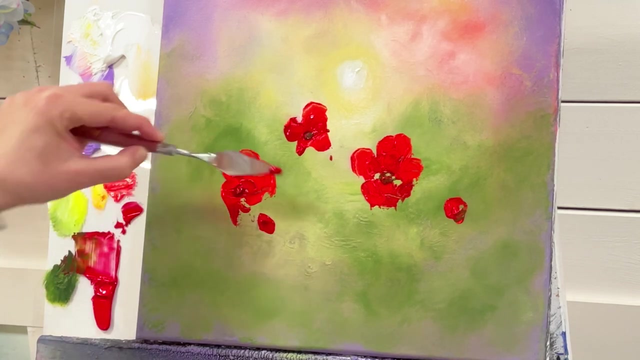 It's like the sun is coming through them. Then I'm going to take a little bit of my sap green, mix it with some red and I'm going to add a little bit inside the flowers. Add some smaller ones and you can layer over ones that are just little buds. 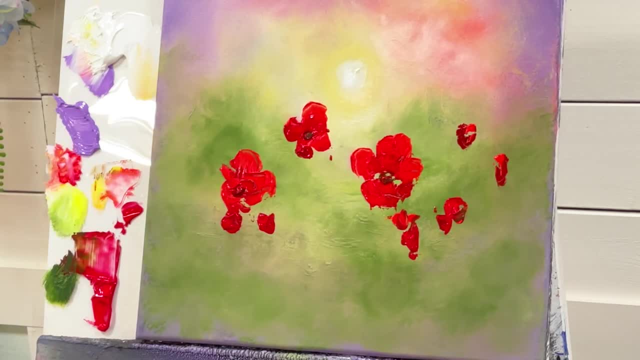 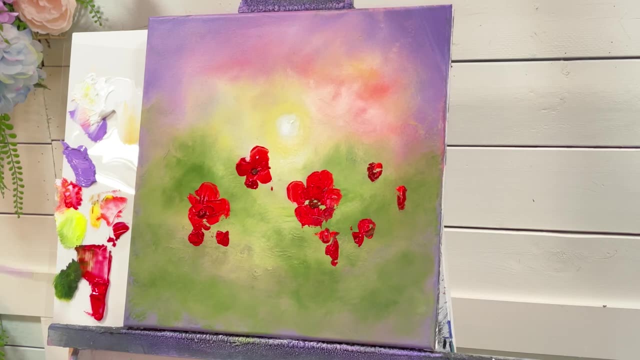 And take my liner brush, add a bit of water to it, Sap green. A little scoop at the base. Let's just add a few little faint ones in here, just picking up more water. I've got lots of paint in my brush. 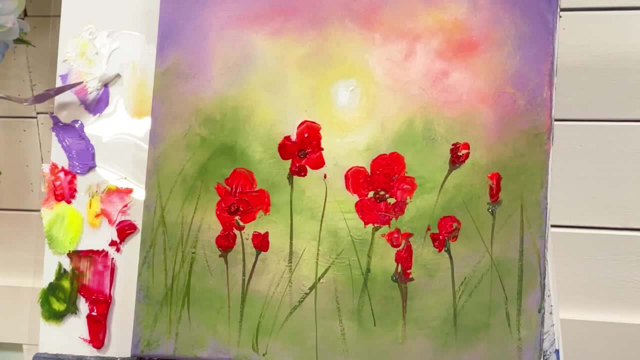 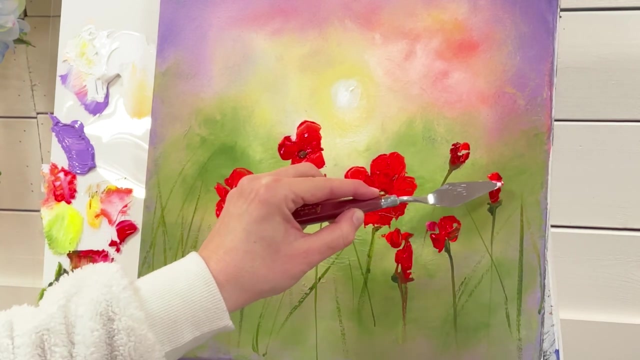 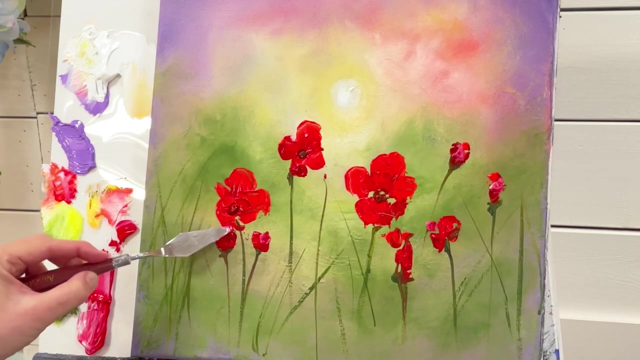 Okay, now I'm going to take a little bit of white with some red, Kind of mix it up a little bit. I'm going to add a little bit of this for a different shade. We could add some other little flowers. I'm not using much of the palette knife. 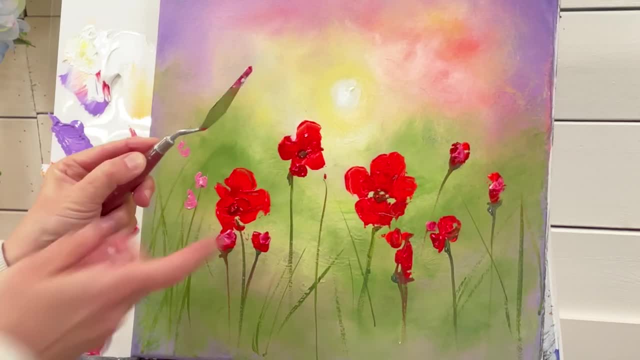 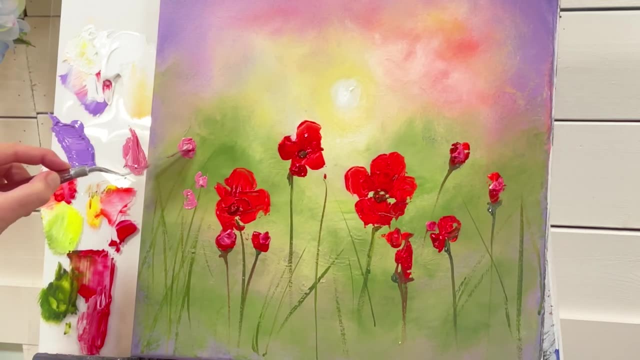 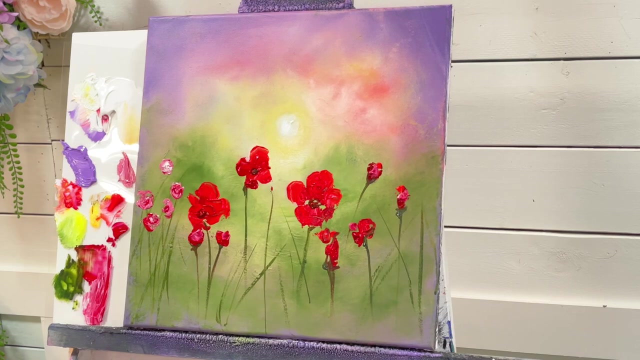 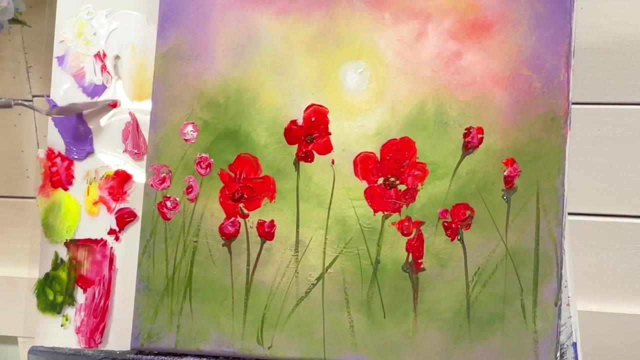 I'm really using the tip there so you can see how much paint I have on there. Okay, we'll take some more of my luminous red, Some white with that, Some red on here, Okay, All right, This is kind of the base I'm going to do. 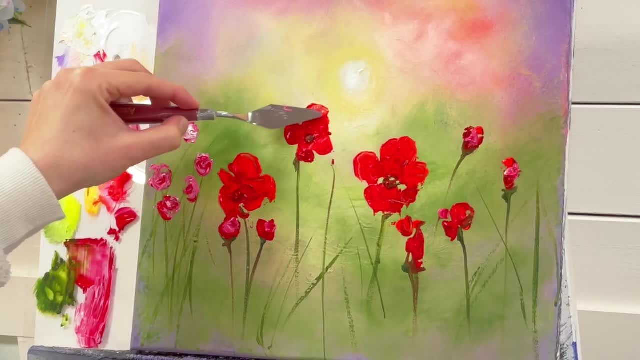 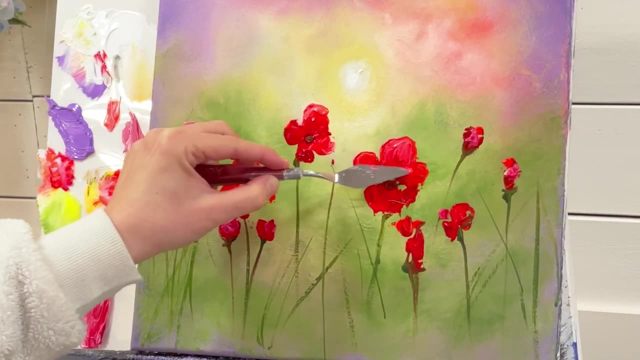 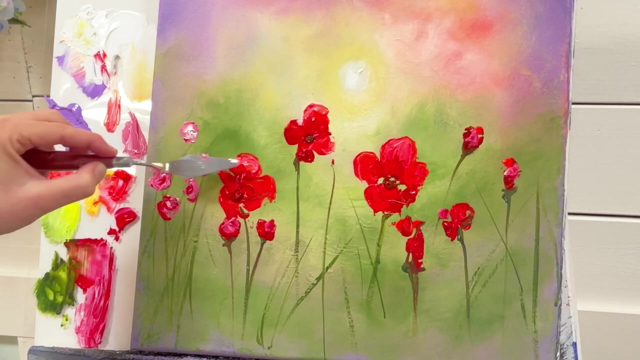 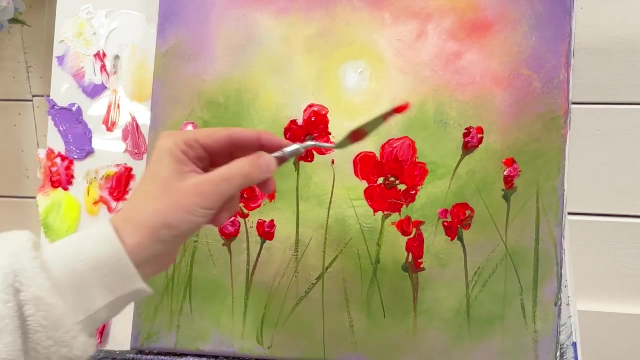 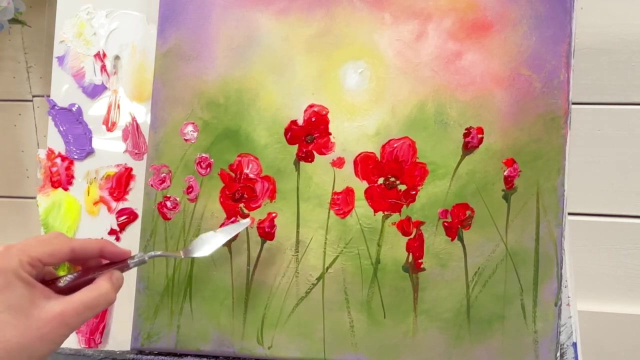 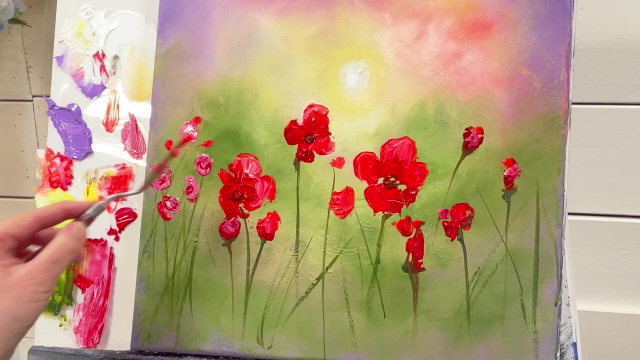 So I'm going to add some more of my paint. Okay, We're going to use some of my paint too. Add some of that inside The petals here that are on the top and the side. There's so many different textures. 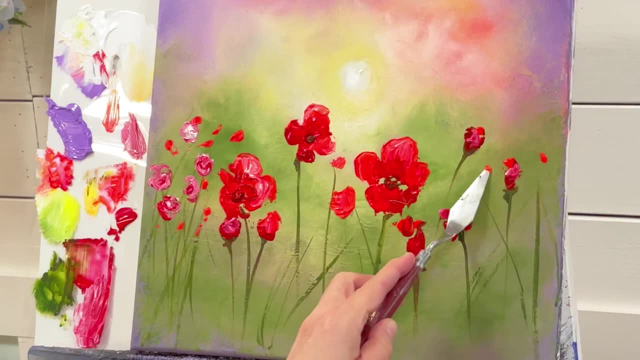 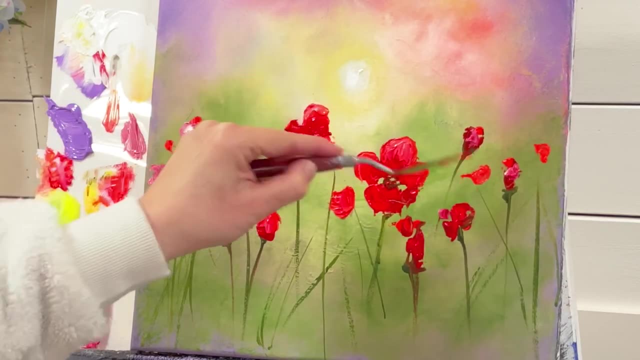 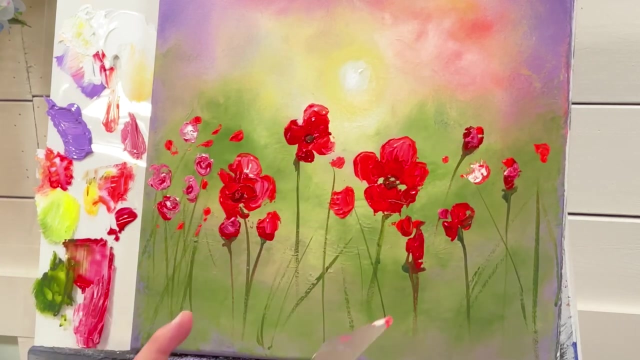 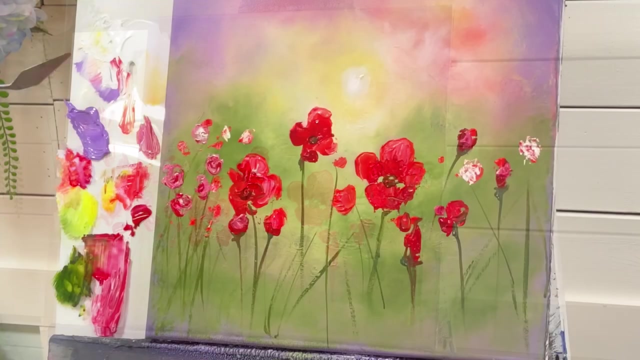 You can get and create different flowers by how you push and tap or gently push and then twist around and take a little bit of white. Okay, let's take some purple. it's okay if there's a little bit of red in there, Some purple and white. 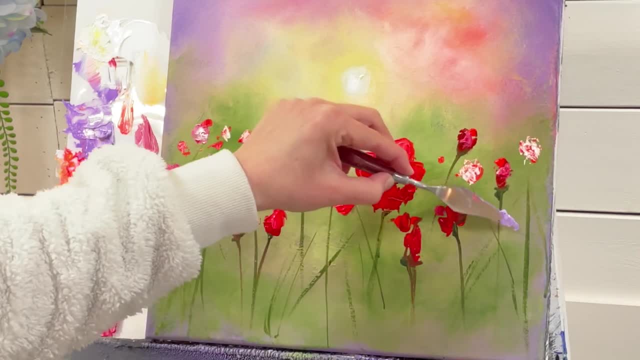 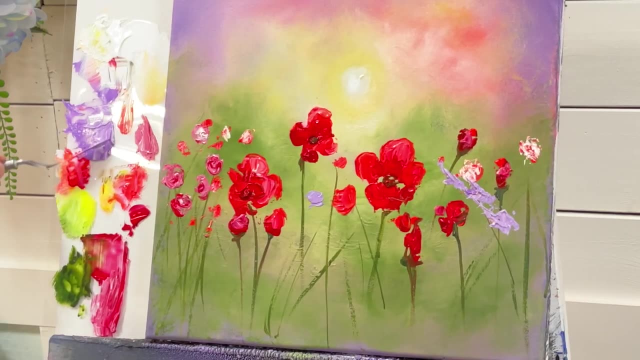 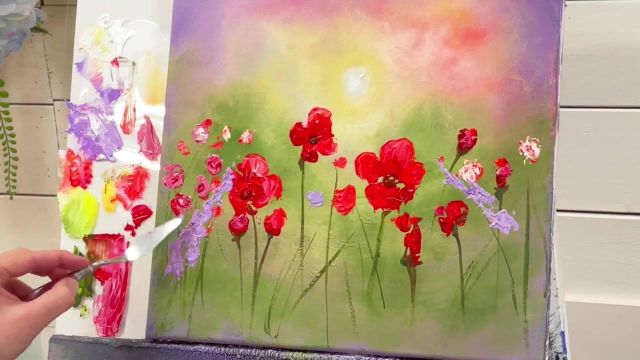 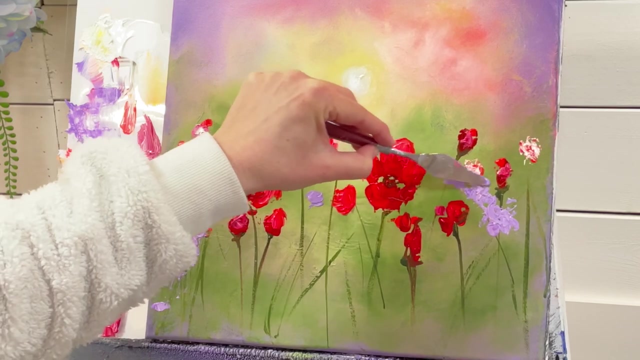 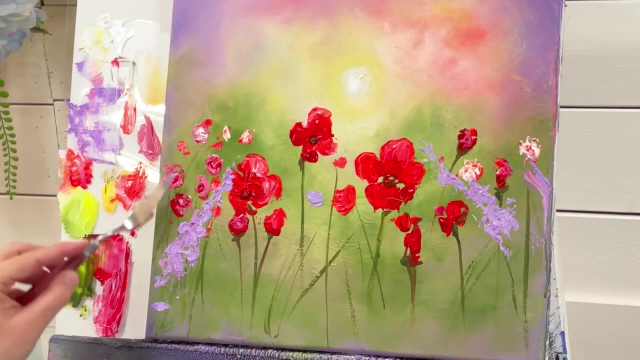 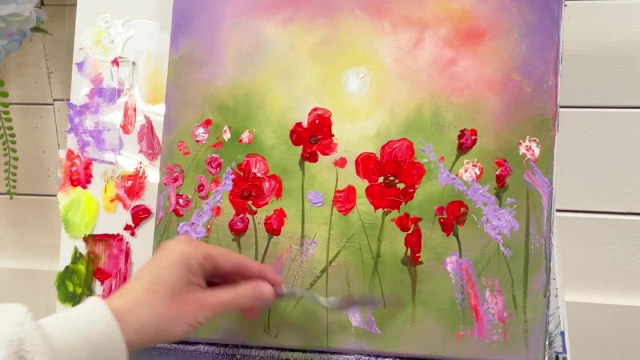 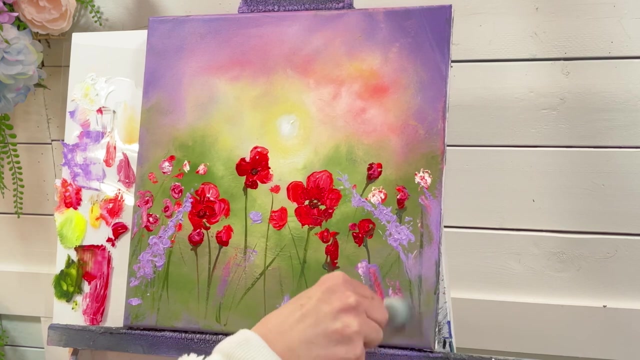 And start adding a little bit, Okay, Kind of like little stalks, flower stalks, Okay, And I'm just going to pull in like this and take another mop brush, tap a little bit and then just soften, Okay Okay. 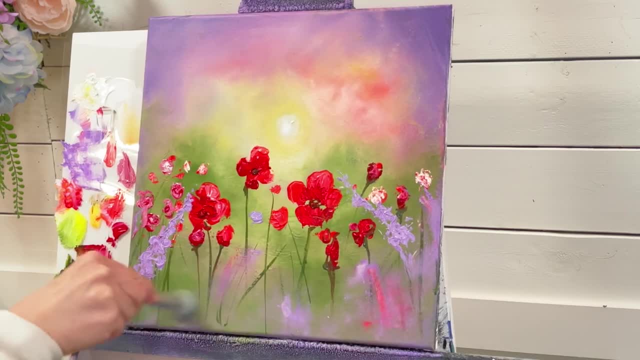 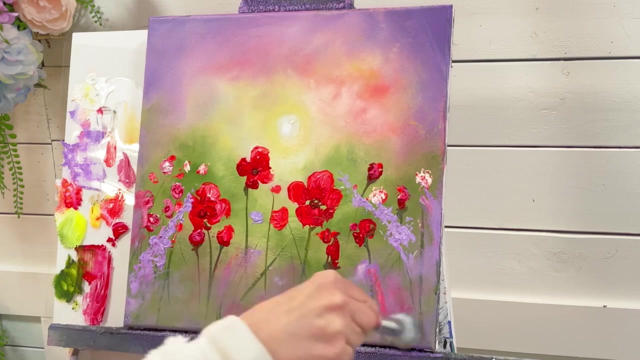 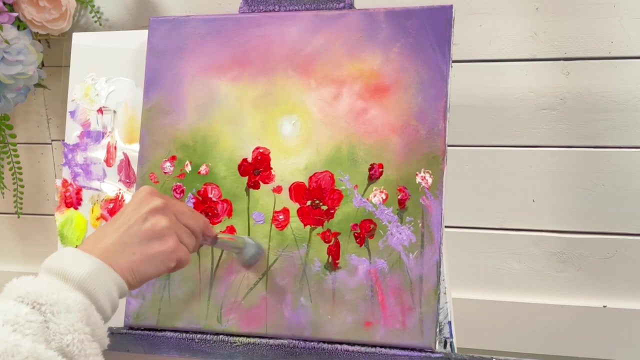 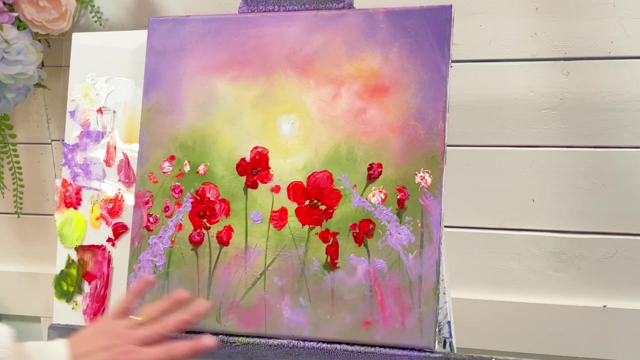 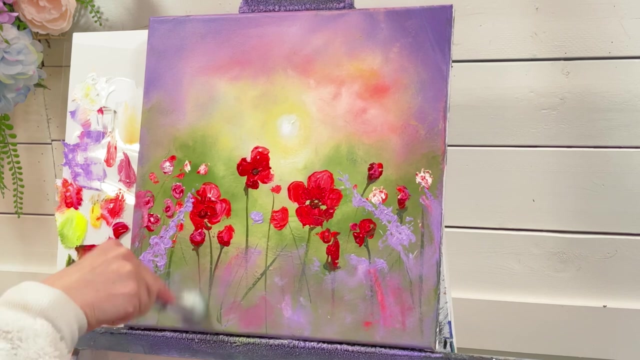 All of that Beautiful. Now I'm going to take a little bit of this yellow and I'm just going to blend it in. Okay, have blurry out of focus here in the in the front, and then our flowers that stick out more, and then soft and out of focus in the back, so you can build it up. 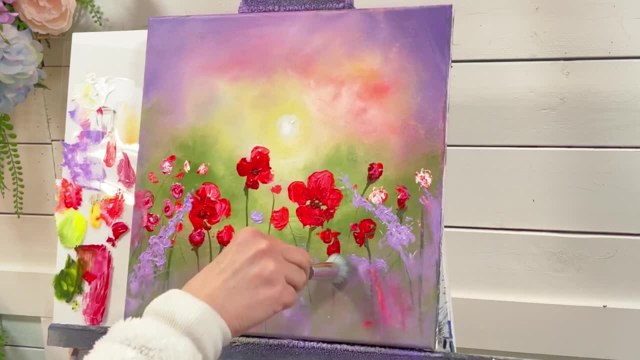 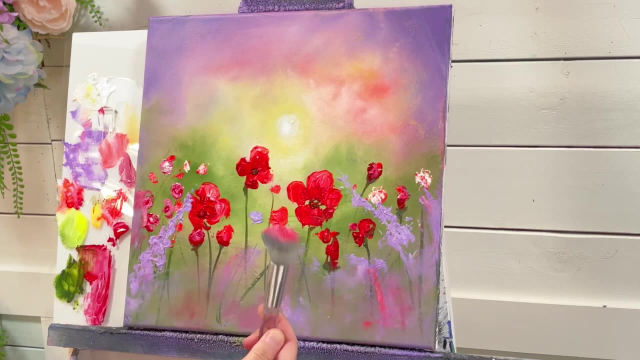 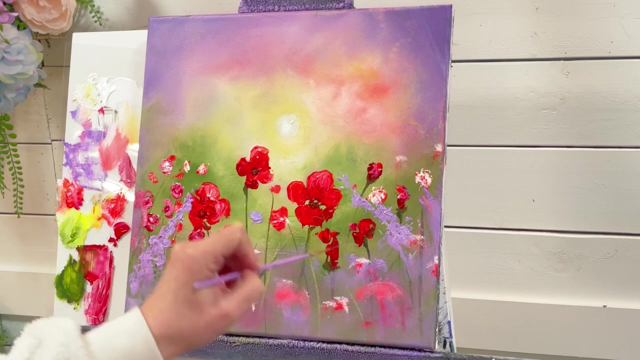 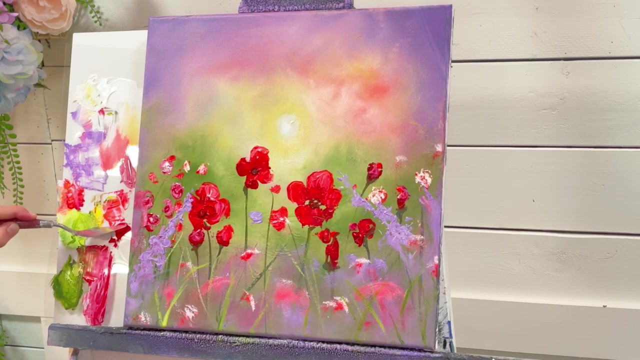 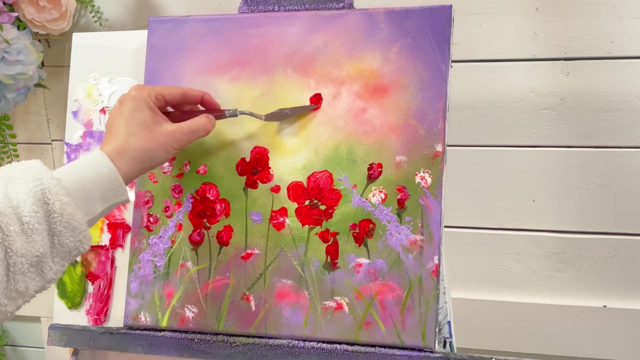 in layers. take a little bit of the paint off some of these areas or add a little bit. i'm going to take my liner brush again: some yellow, some green and some white. okay, Add some stems that stand out a little bit more. Okay, I'm going to take some more reds- both of my reds here- and I'm going to add a larger. 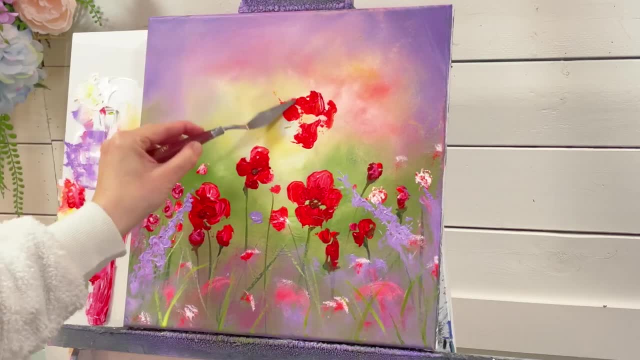 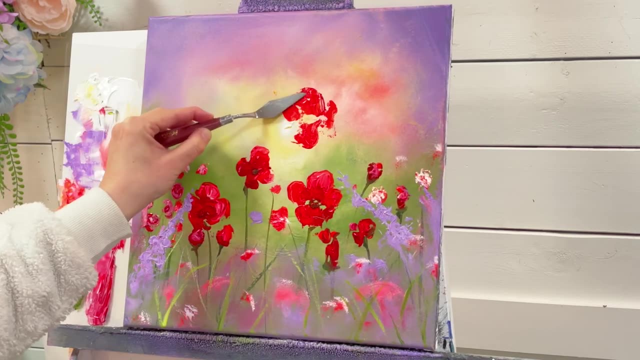 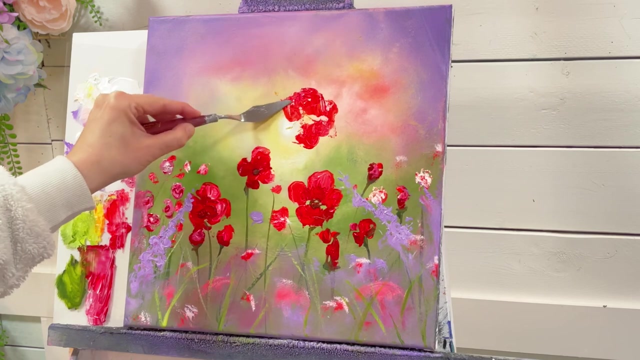 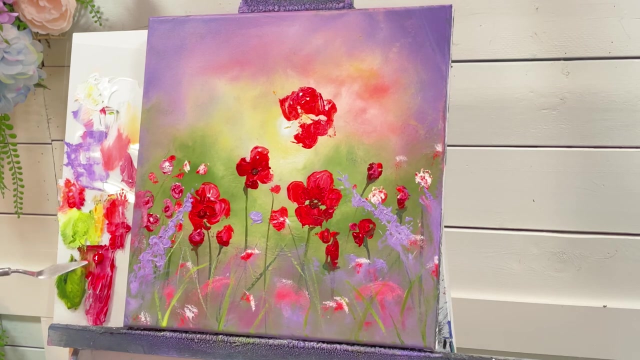 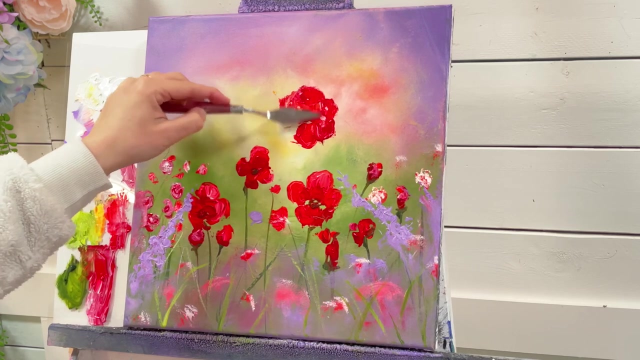 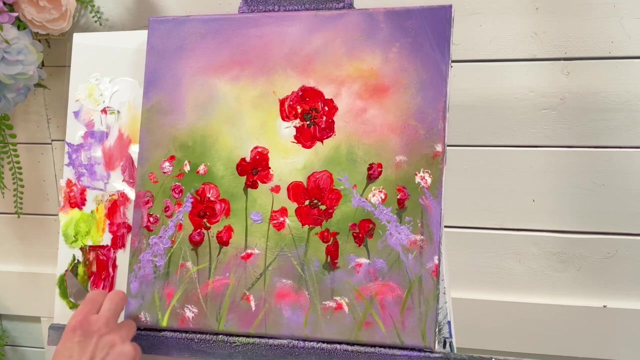 flower right here. There we go. A little bit more of my sap green. I'm just going to take red for now, though. Okay, there we go. Okay, now I'm going to take the green and dab that in the middle. 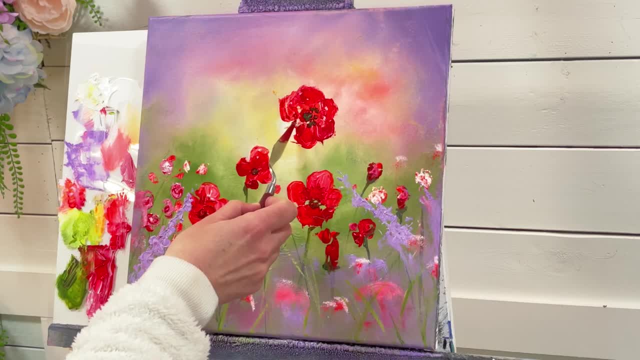 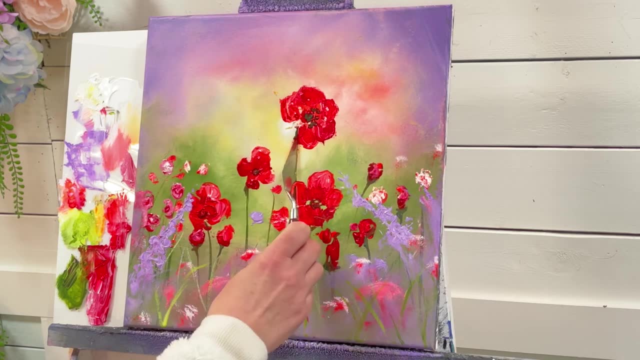 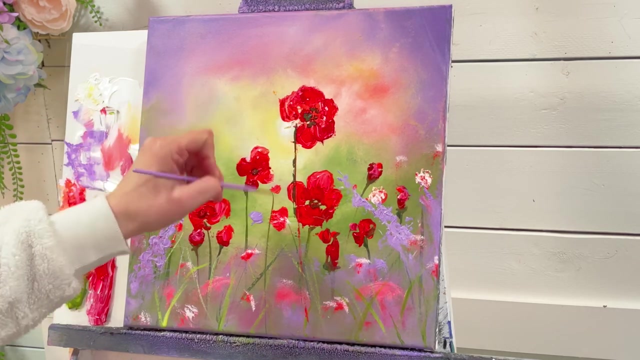 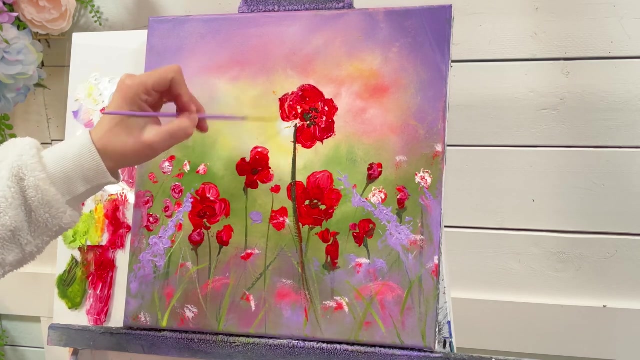 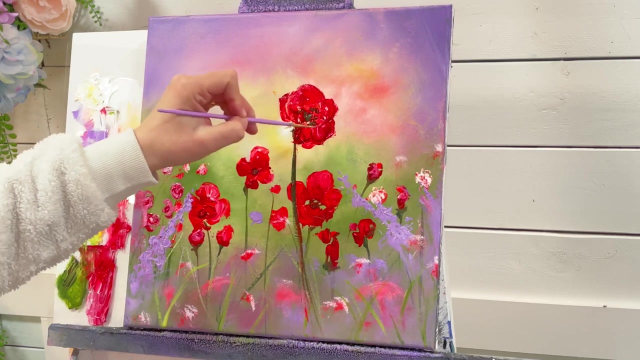 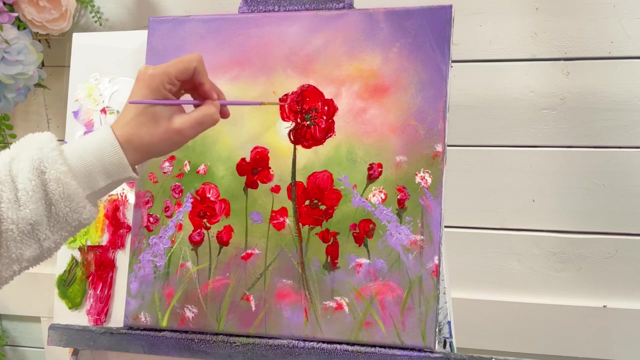 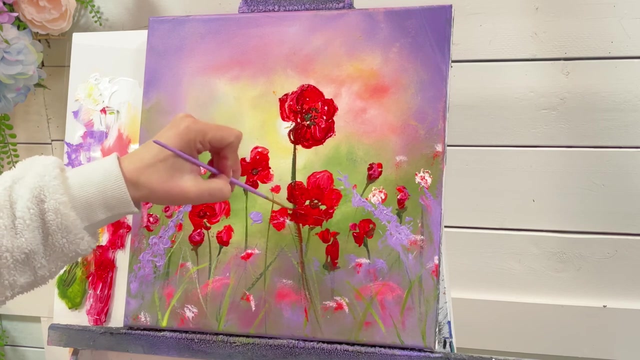 Take a little bit more Down on our left. Okay, Give it a little bit more of an angle Now. with a liner brush, I'm just going to blend some of this green in with the red to make a darker shade. Okay. 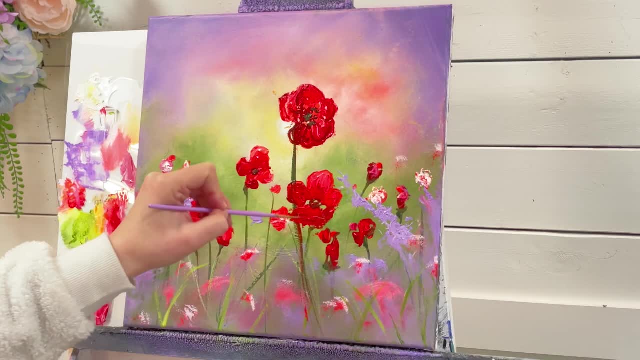 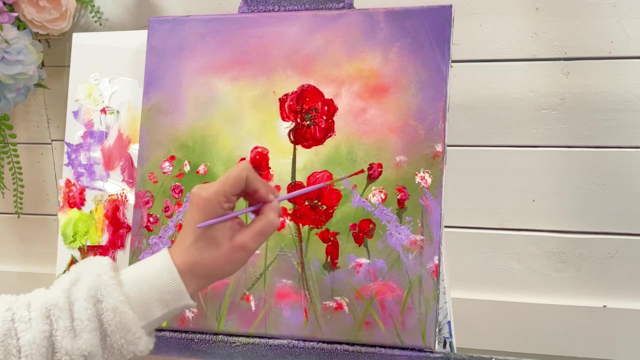 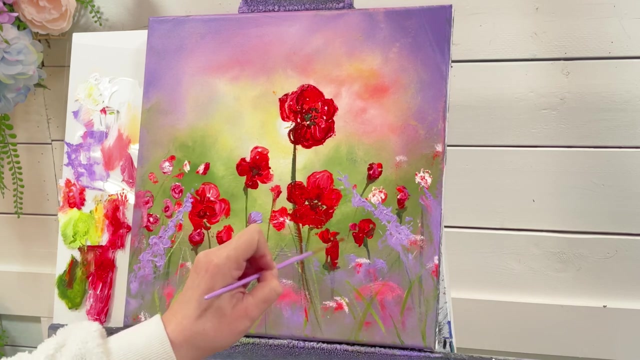 There you go, Alright, Okay. so now we're going to take our pink and we're going to put this one here, right here, And we're going to just smooth that down. Okay, Okay, Alright. So there's still lots of paint in my brush. I can use that. add a few other darker flowers. 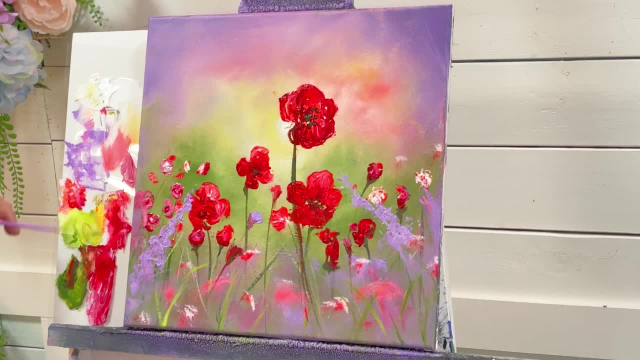 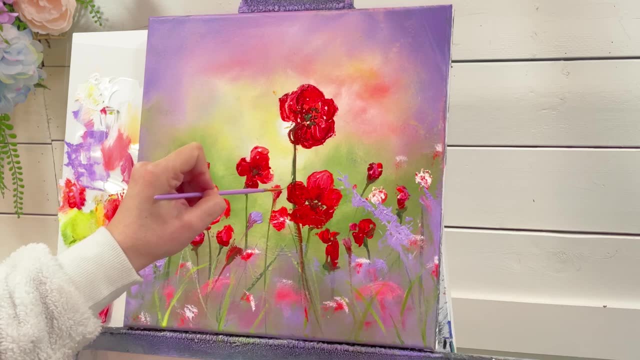 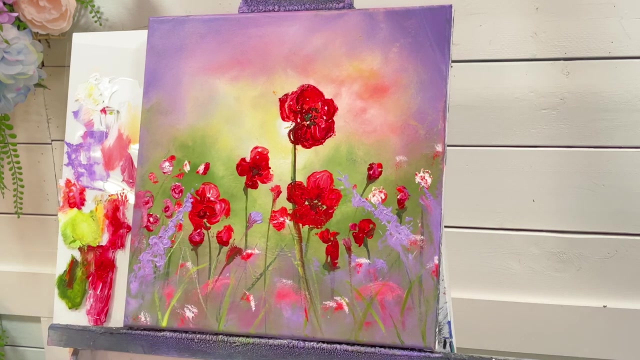 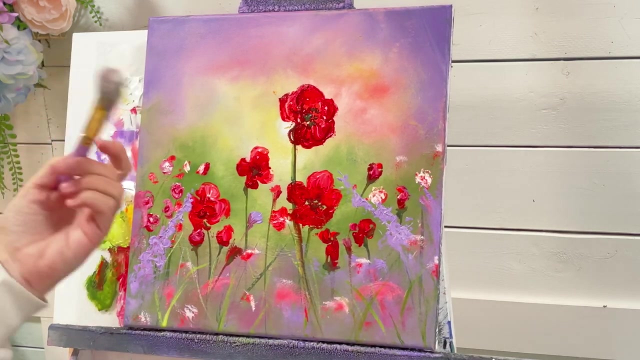 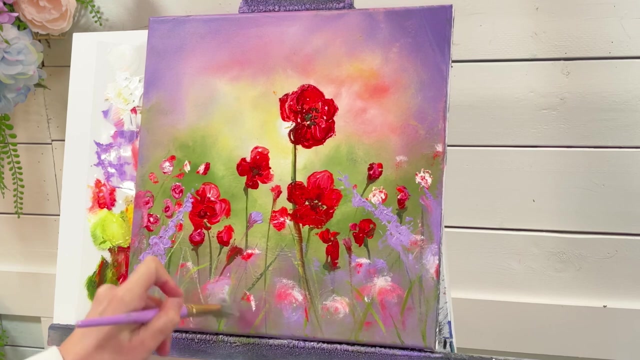 I'm going to go into my light green here. a little bit of white. I'm going to soften some of these flowers. take a little bit of white, Okay. Okay, You can twist with your brush to make it look like very soft flowers. 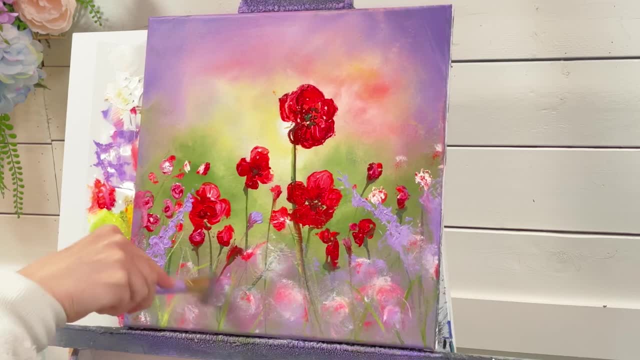 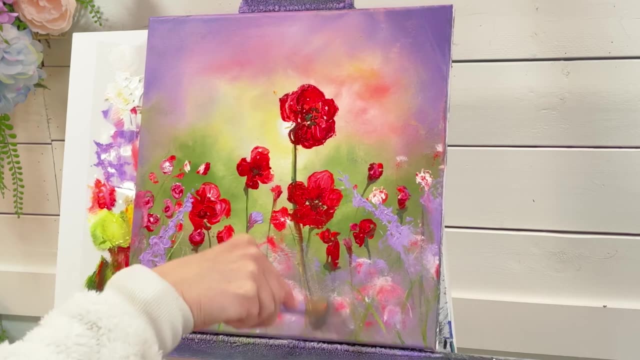 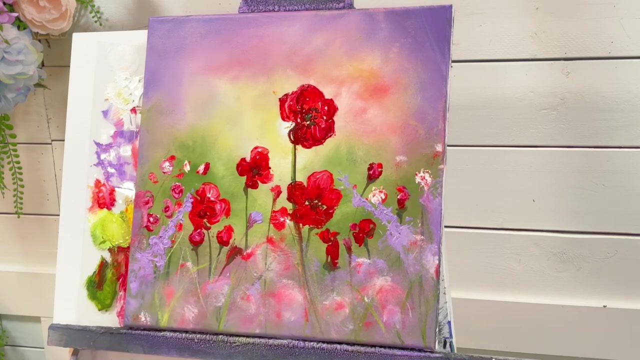 Or you can just go around with a brush. Okay, You can twist with your brush to make it look like very soft flowers. Okay, I'm going to go ahead and go around with a brush to make it look more soft. Okay, I'm going to go ahead and go around with a brush to make it look more soft. 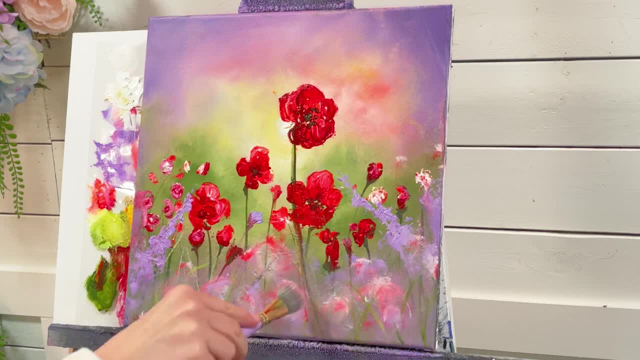 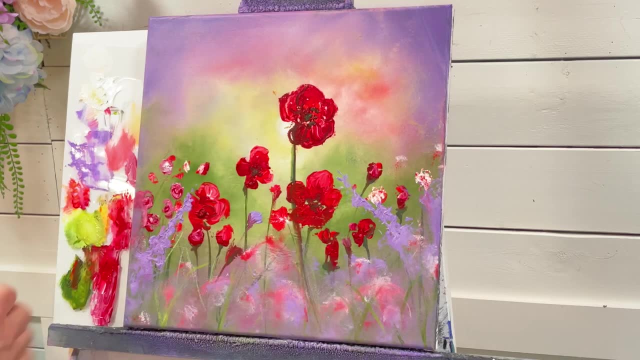 I've got a lot of purple here. I'm just gonna steal some of that and dab it down here. Okay, so I dried most of this off in this area here because we're going to add some sun rays, I'm also going to add a few more flowers down here, with some pink and orange. 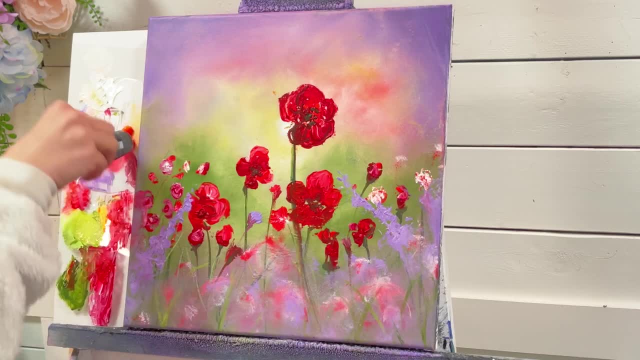 So I'm going to introduce a couple new colors. I've got luminous orange here, So I'm just going to add some right there. I'm also going to add a little bit more of my neon red, And I'm going to add some luminous opera. 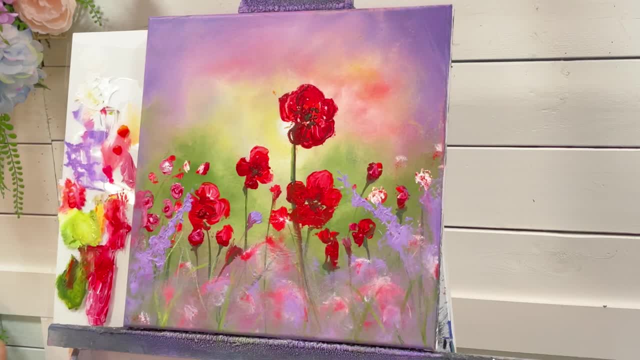 Okay. neon pink: a little bit right there, okay, so i'm going to be using a small flat brush. any small flat brush will work. you can have one a little bigger than this or even a little bit smaller, and i'm going to get my brush a little bit wet. okay, so i've got luminous lemon, yellow, neon, orange. 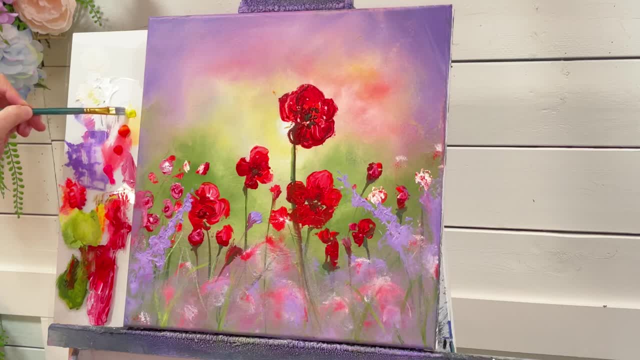 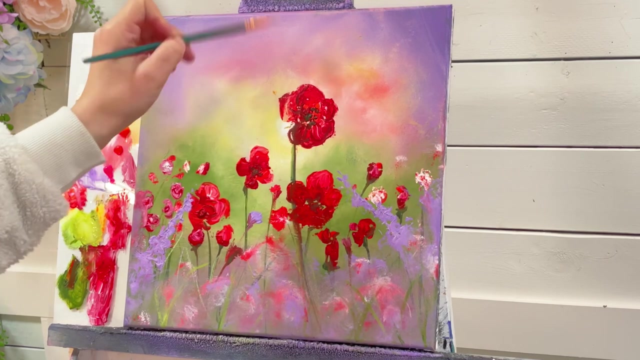 neon red and neon pink. a little bit of water, a little bit of yellow. i'm going to take a little bit of orange. we get this really soft, beautiful peach color and we're gonna- the sun is right here, so we're gonna just add some sun rays right over this. 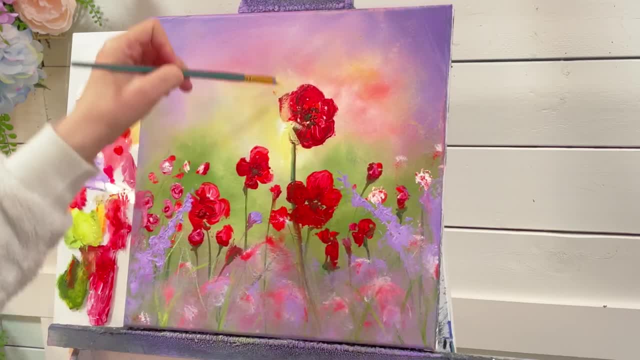 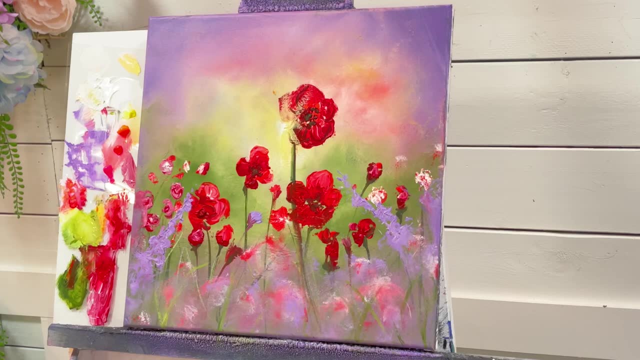 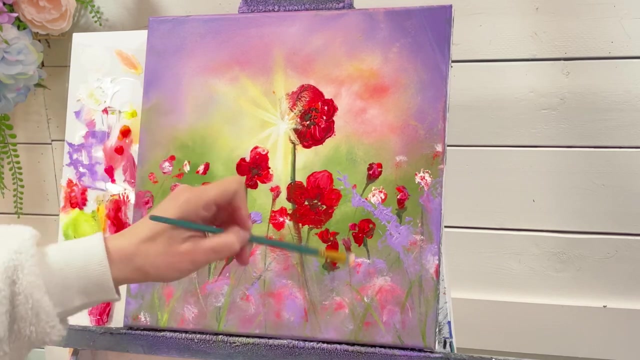 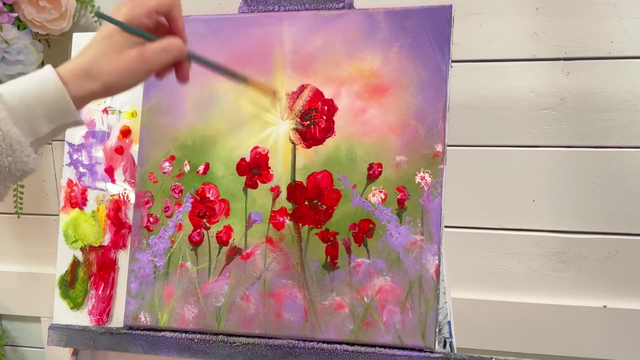 just gently pull down, add a little bit of water if you need to add a little bit more white, right in here, gentle little flick shorter flicks a little bit more of the orange, a little bit more yellow and white, so now it looks sparkling. if you pick a little bit of the red up from your poppy, that's okay. 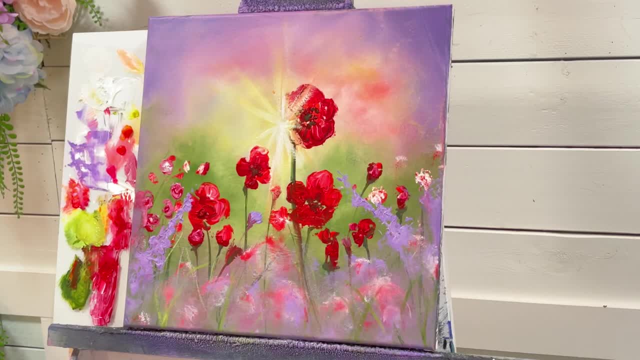 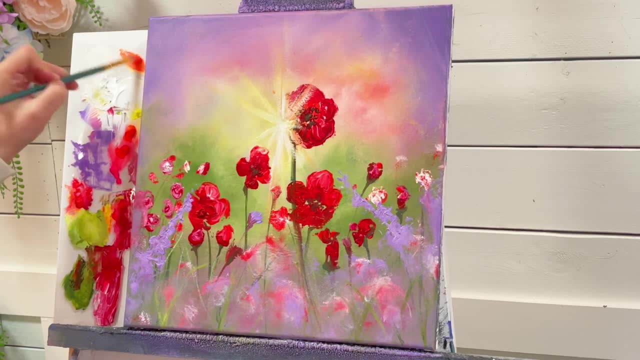 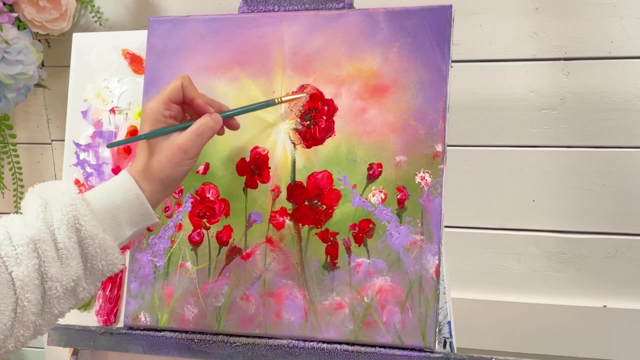 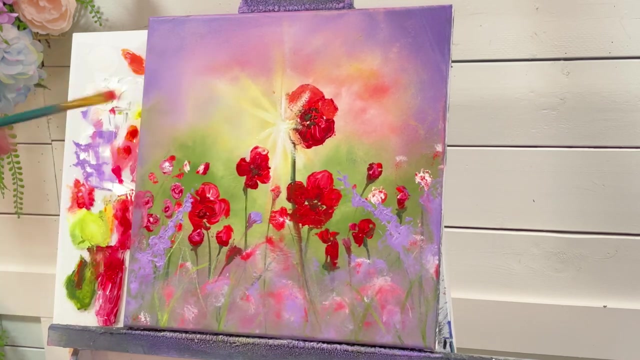 kind of just looks like it's in the in behind there anyways. okay, so i'm going to take a little bit of orange and red now, mix that with my peachy color and i'm going to add inside some of these petals. my orange will have a dark berry. I'm going to mix my black eye color. 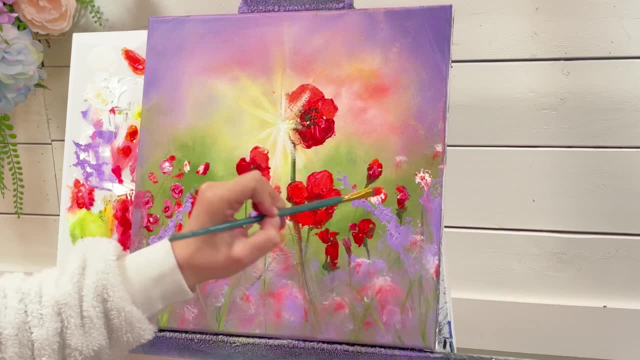 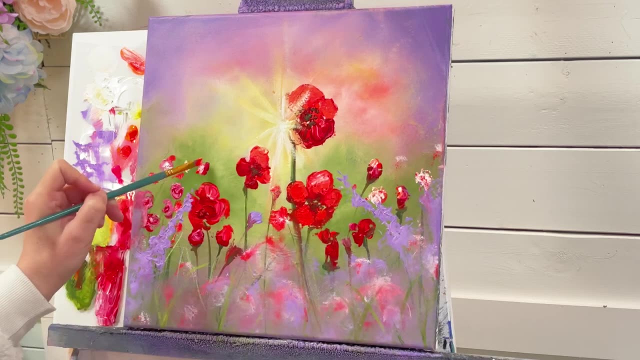 into my iris, uh, and then, when the artificial 오빠 hair's done, add a little bit of white. I'm going to add some flake on the tip of my eye, or whatever you want to call it. it really just tries to outshine the skin. 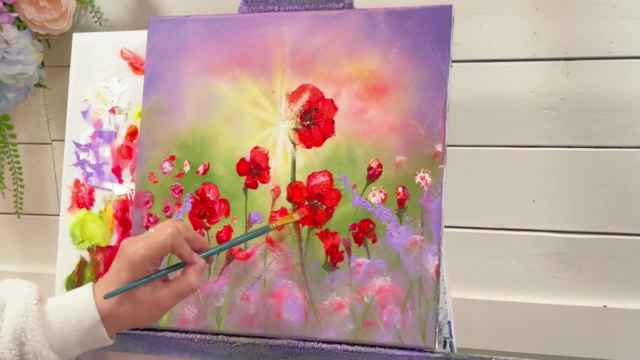 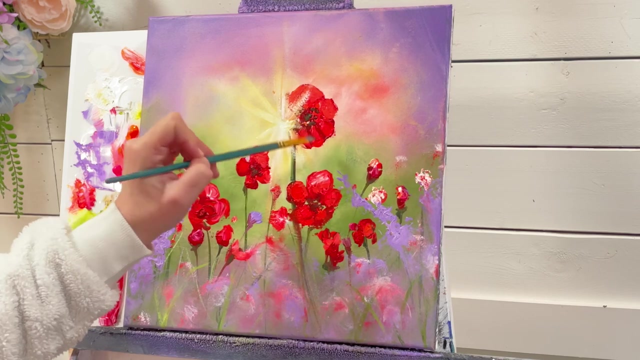 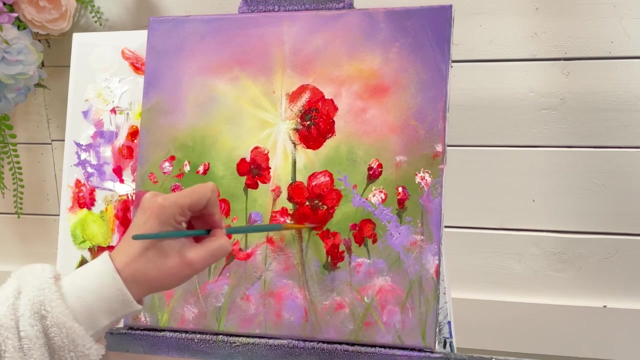 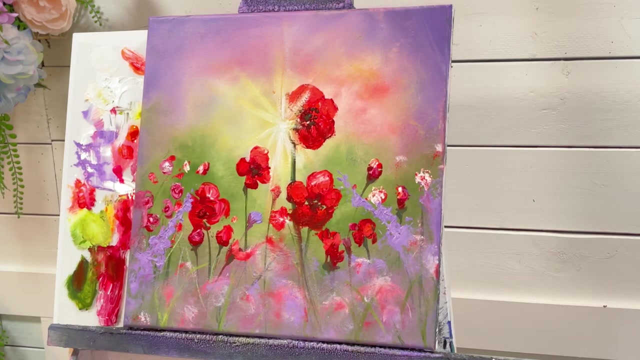 my Let's go ahead and take a little bit of our Natphal Crimson and our green, add a few darker shades of red in there. and let's go back over to our palette knife now and take some pink and some white And just add. 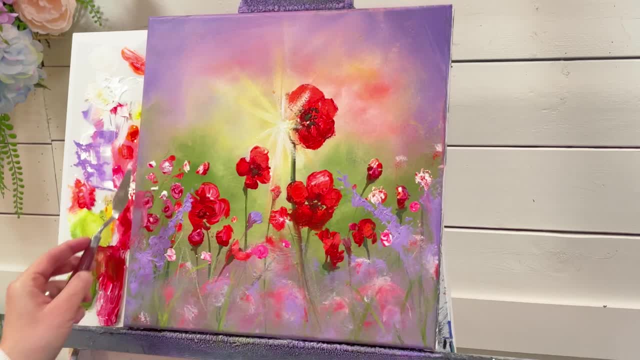 some little dabs for some small flowers. I'm going to add a little bit of yellow with white on top right there, but here as well, anywhere we want to have the sunlight hitting. Take some orange, pink, yellow and white. 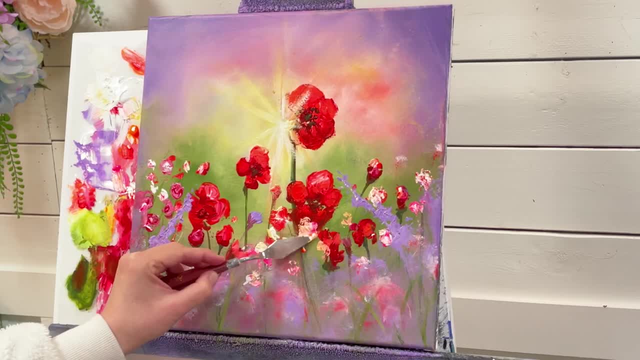 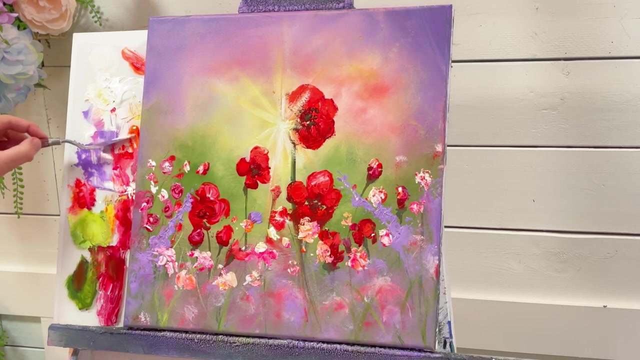 Don't be afraid to layer over some of those other flowers. You want that layered look. This is just one of those really fun abstract types of paintings where nothing looks realistic about it but we just get this sense of beautiful summer light hitting these wild flowers. 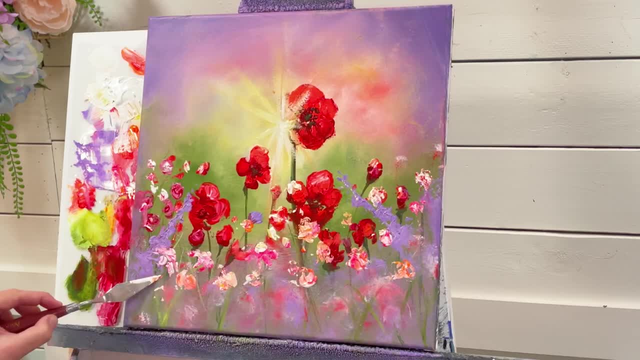 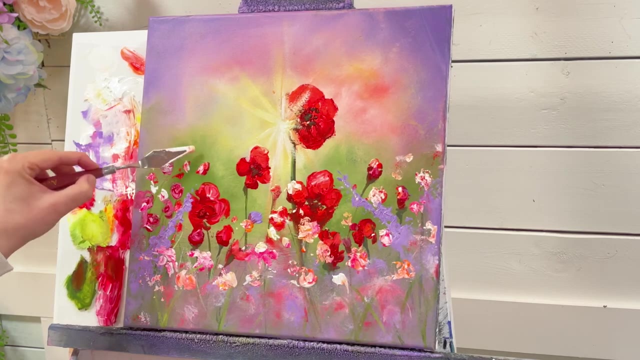 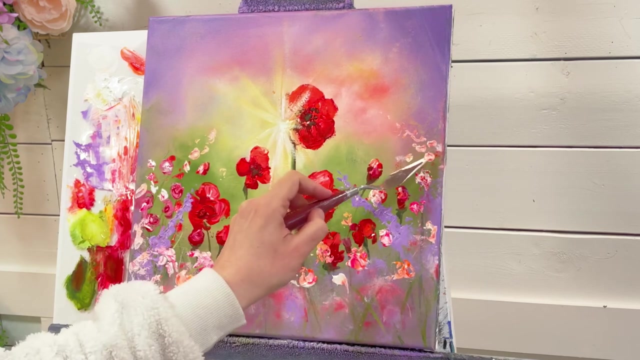 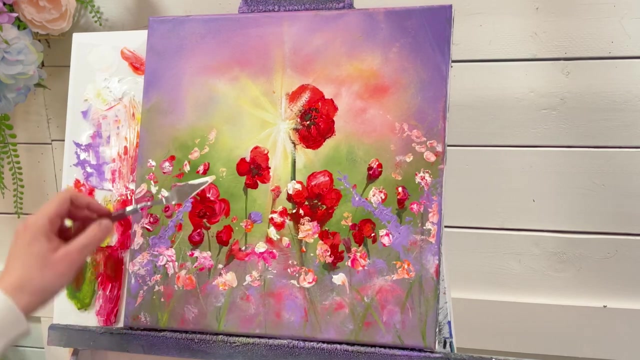 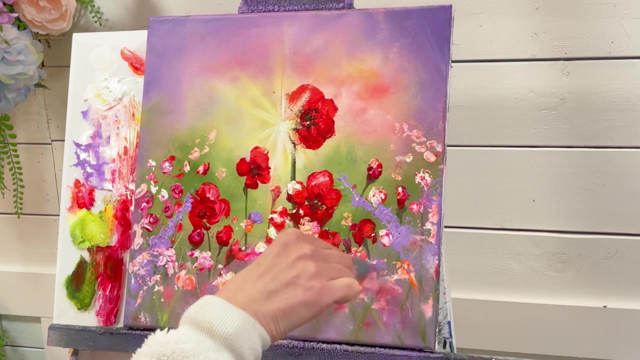 whatever I've got left. here I'm just kind of putting on my palette, pushing slightly, mixing. I've got another dry mop brush here. I'm going to go ahead and do that here. I'm going to go ahead and do that. here I'm going to catch some of these flowers that are a little bit wet still. 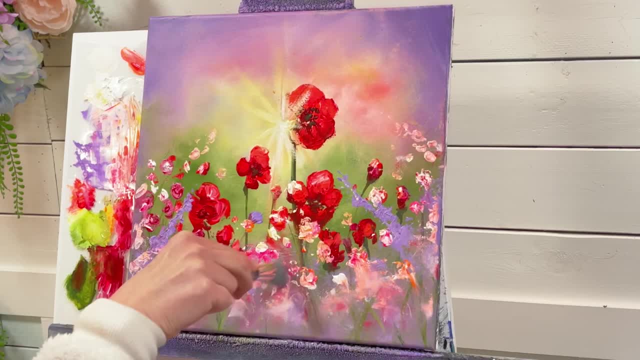 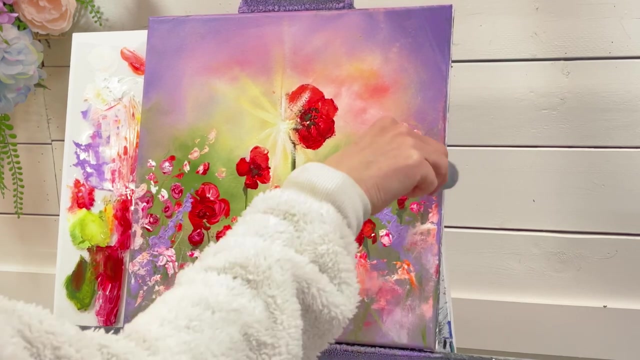 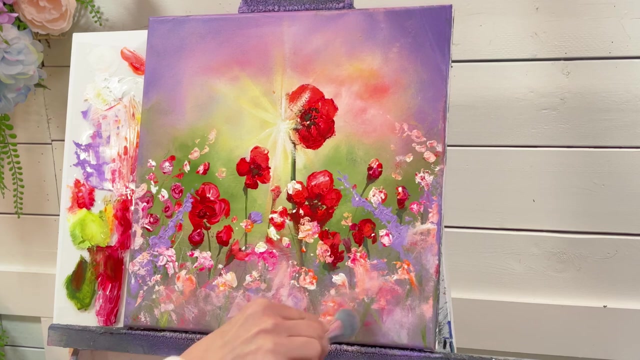 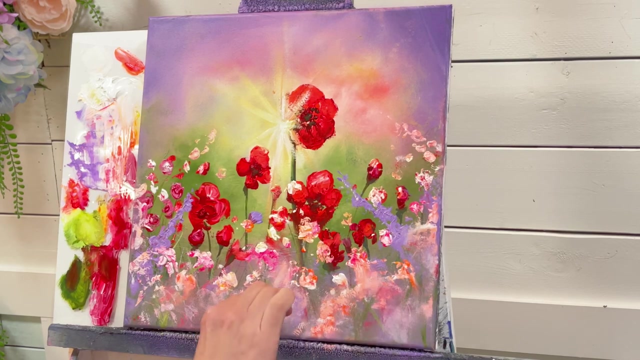 soften, soften. take a little dab. take a little dab just on the end of my brush here. a little bit of that peach. okay, I'm going to take a little bit more of my sap green. a little bit of water. okay, I'm going to take a little bit more of my sap green, a little bit of water. 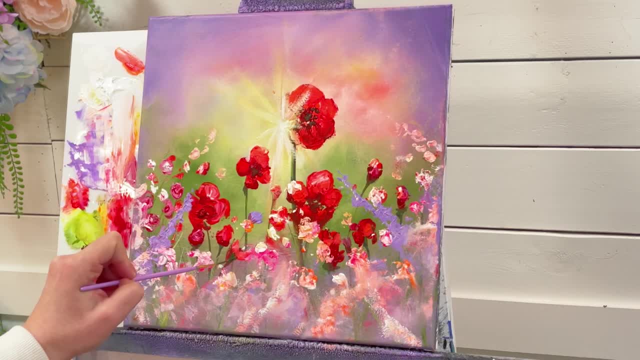 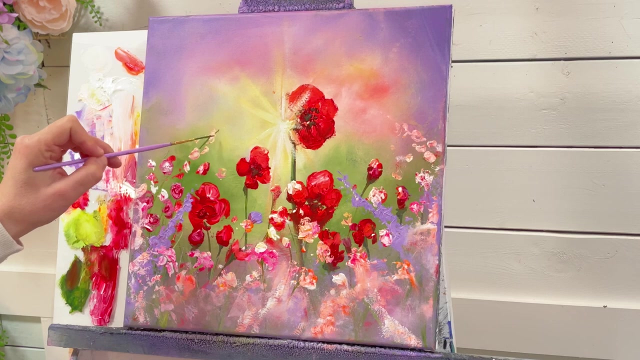 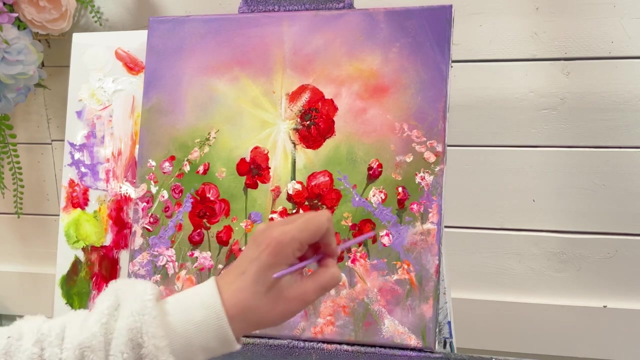 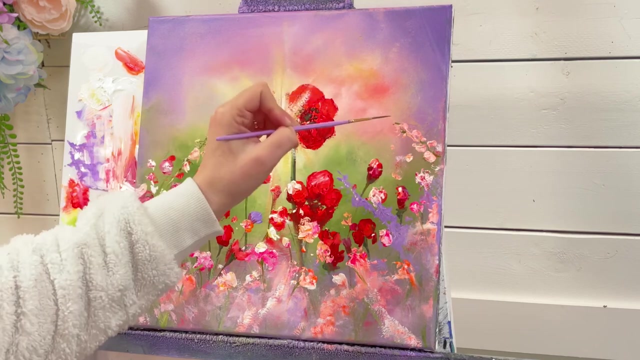 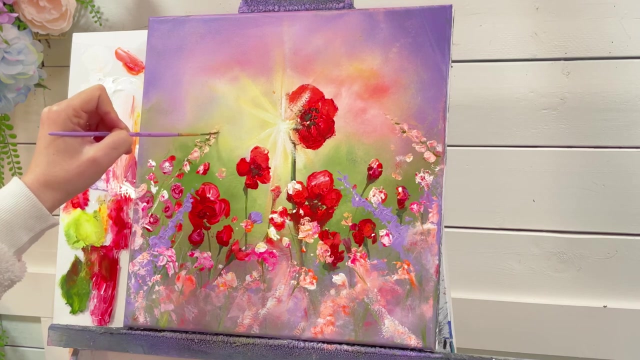 okay, I'm going to take a little bit more of my sap green, a little bit of water liner brush and pull some little stems in here. let those colors just pull out and blend. let those colors just pull out and blend. let those colors just pull out and blend. 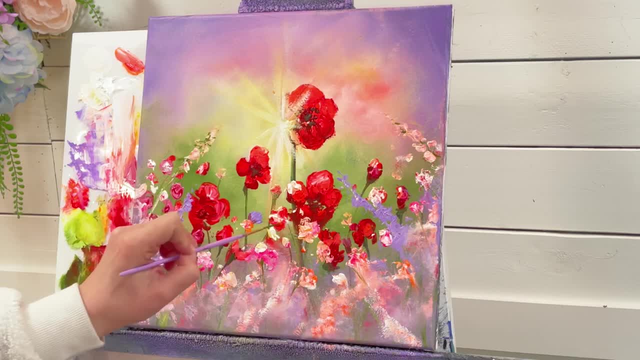 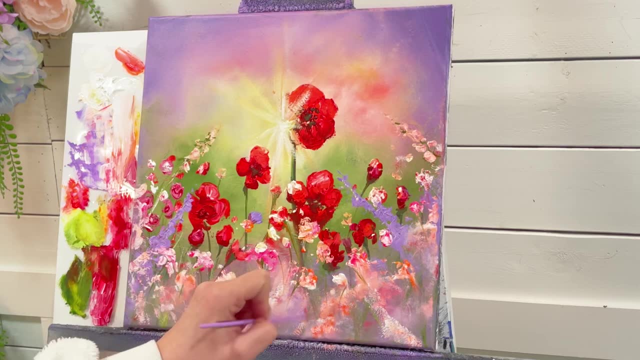 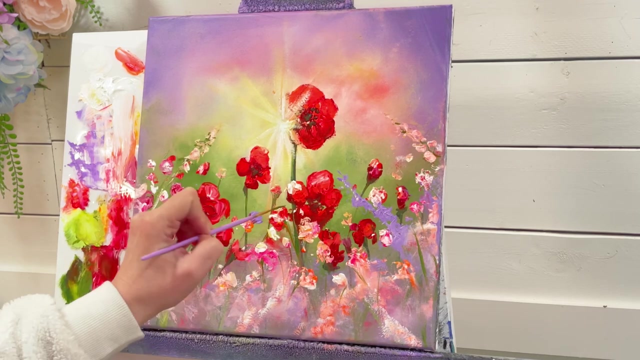 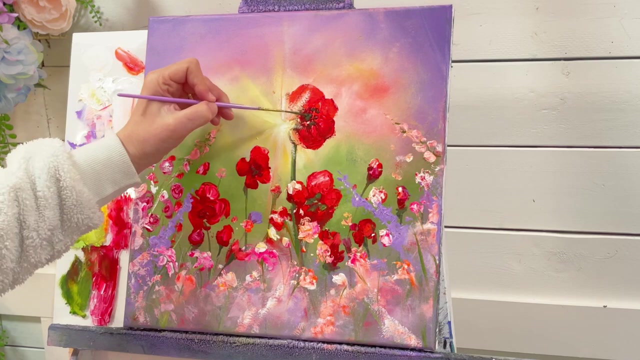 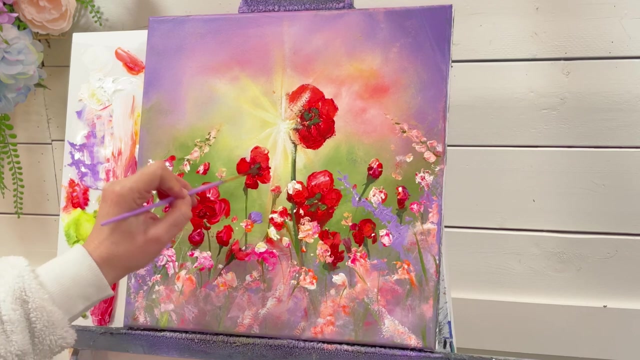 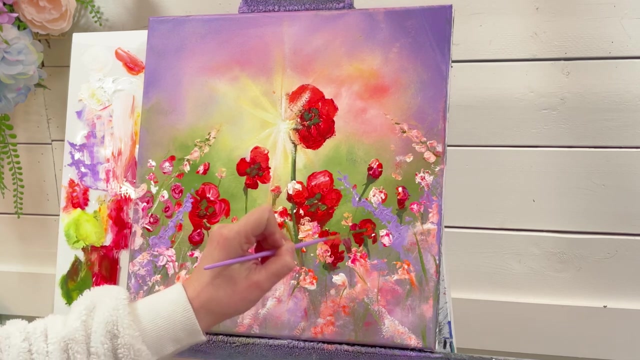 just a little one right back there. just a little one right back there. just a little one right back there, over here, over here, over here. a few little dabs inside the flower petals with green over the red. it'll dry really dark and look black. i've got a glove here. i'm going to do a little bit of finger painting. 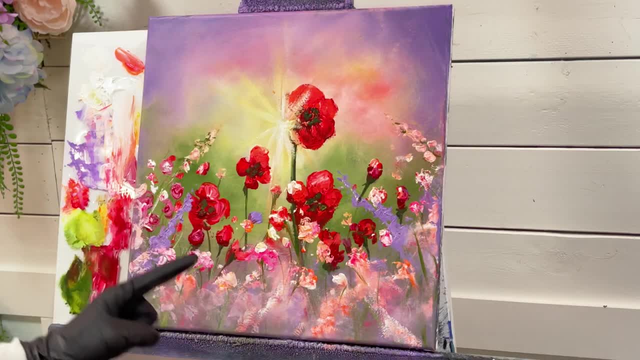 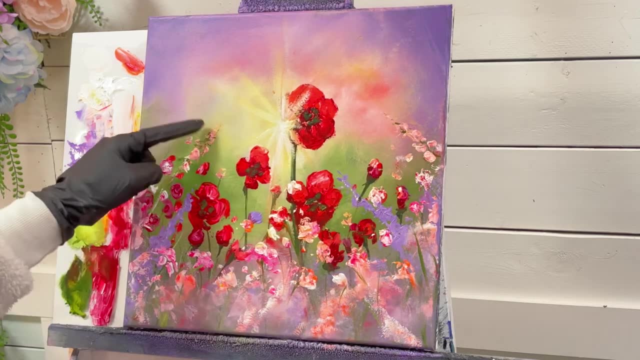 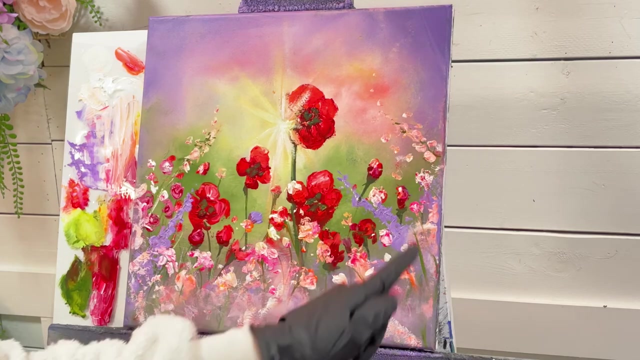 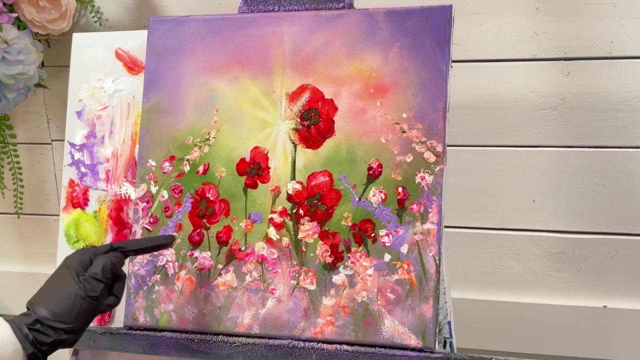 i think that will look really pretty. so i'm just going to take a little bit of the color, the paint that we have here, take a little bit of that off, dab, dab, just little petals like this, and whatever. i've got here a little bit. it's nice when you apply the paint really thick like this, you can go in. 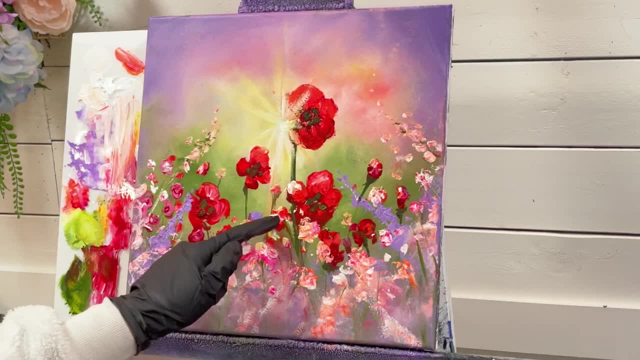 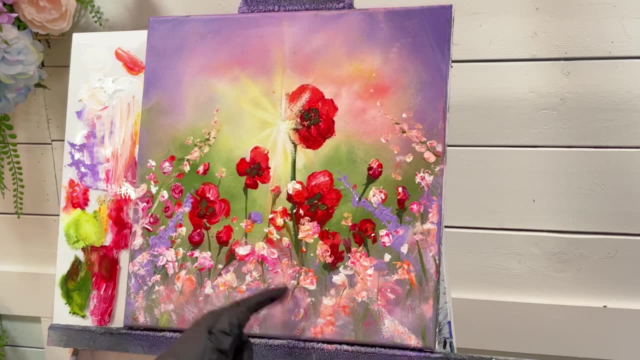 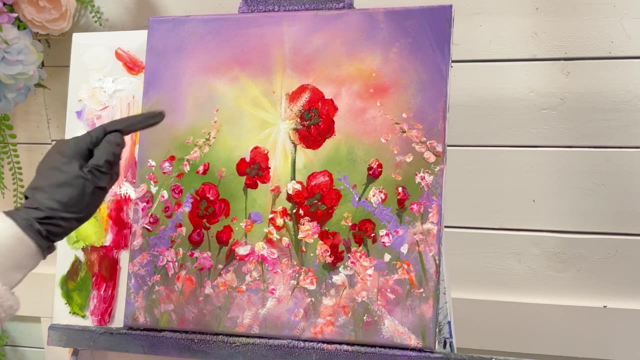 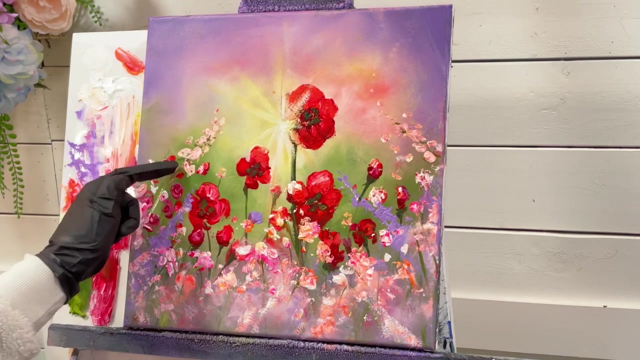 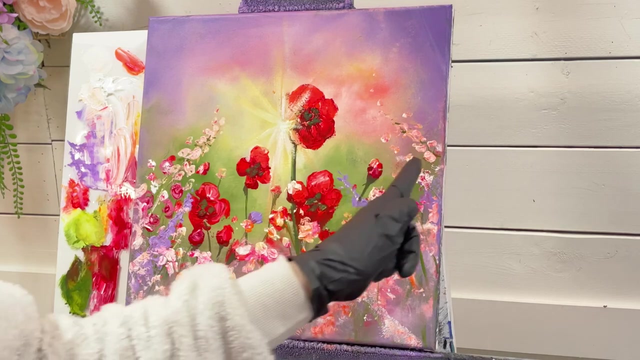 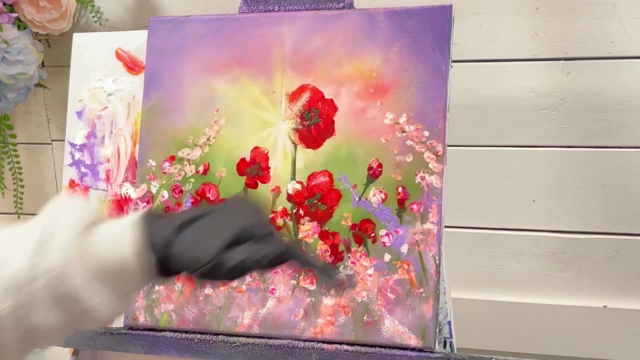 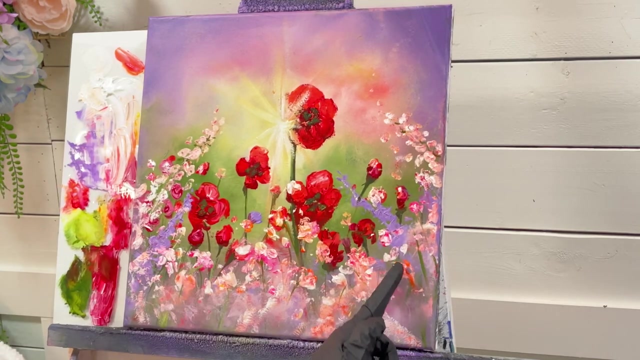 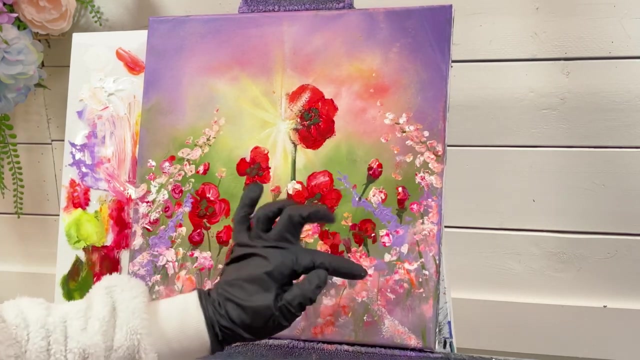 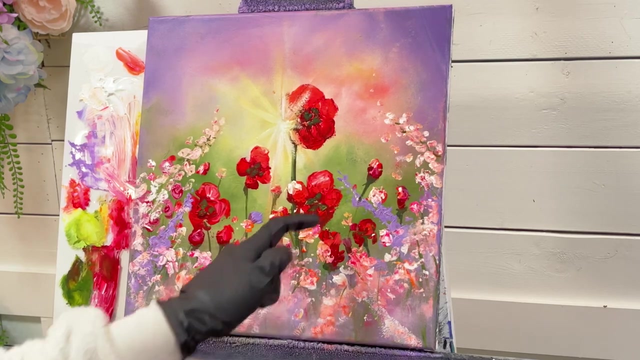 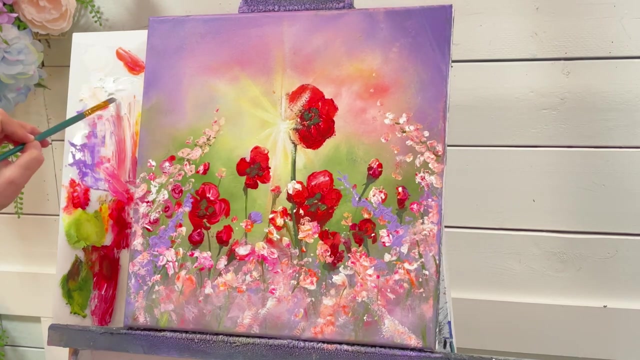 and tap over some of those colors like it's really thick, and then you can use that. it's look like little fox gloves, especially here, how it kind of left a hole like darker center. I'm going to add the final sun rays here. I'm going to go back into my white and I'm 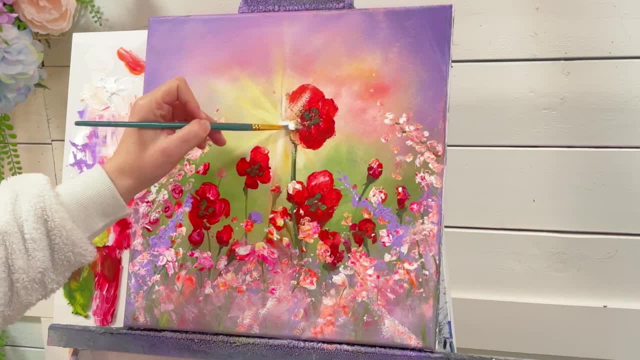 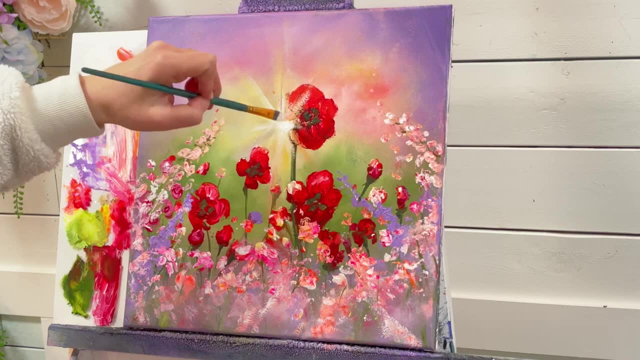 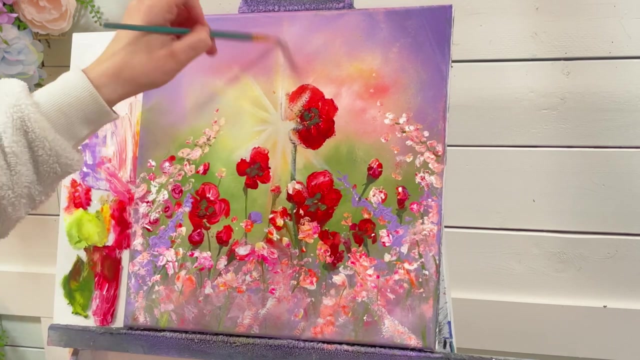 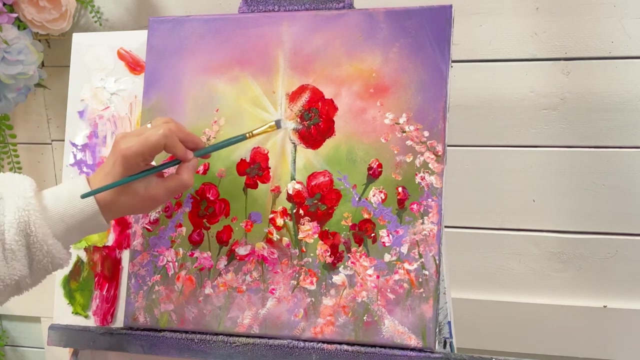 going to go in the middle. make that really bright again, flick. so we're not going to add sun rays over top of this flower, because the sun is kind of like right in behind this. so these petals are in front. you just want to have the sun rays. 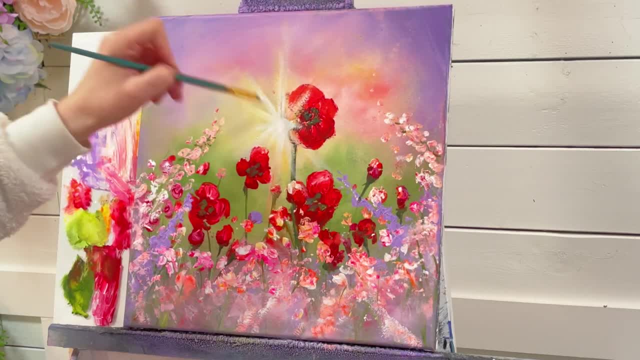 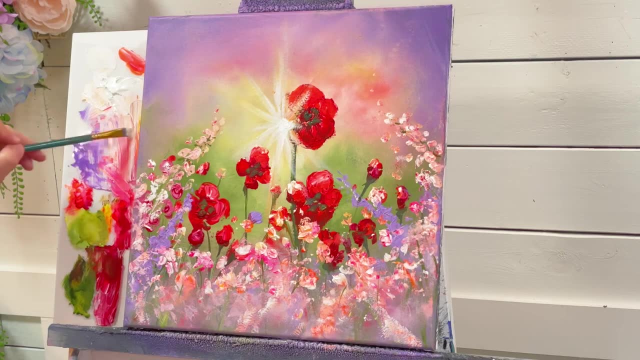 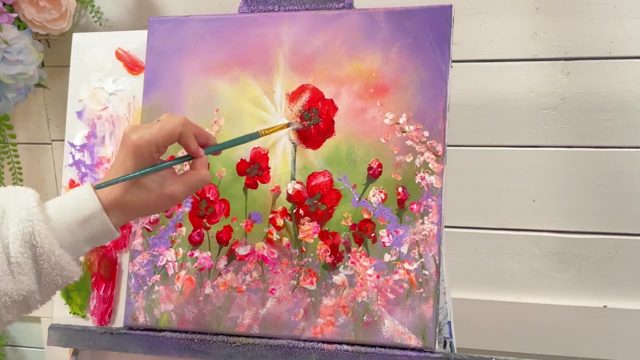 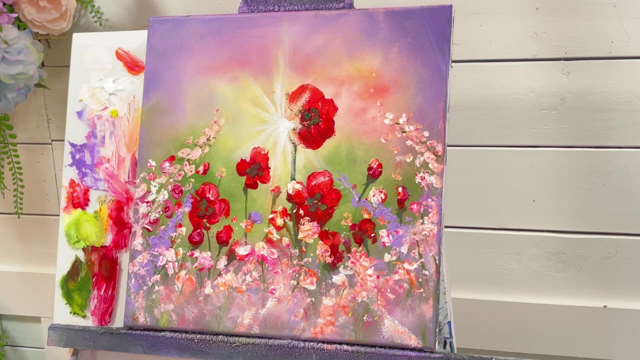 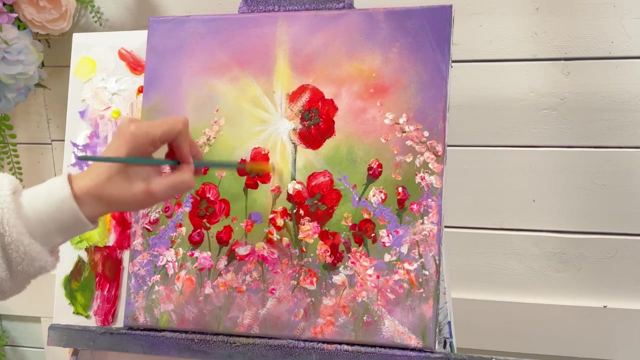 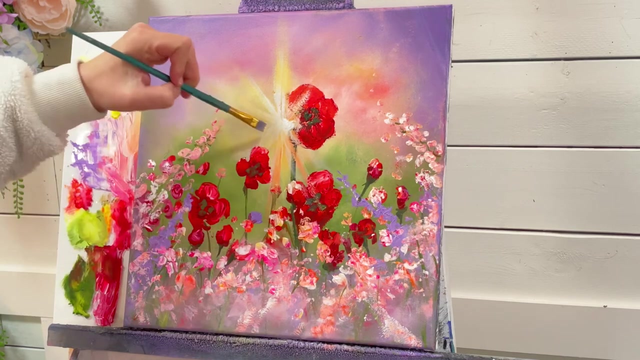 in. Right here, take a little bit of my peachy color, a little bit more, a little bit more yellow. A little bit more of the orange. Okay we look on the same beach, 되 � IT가 되어돌 Spreader pastel. 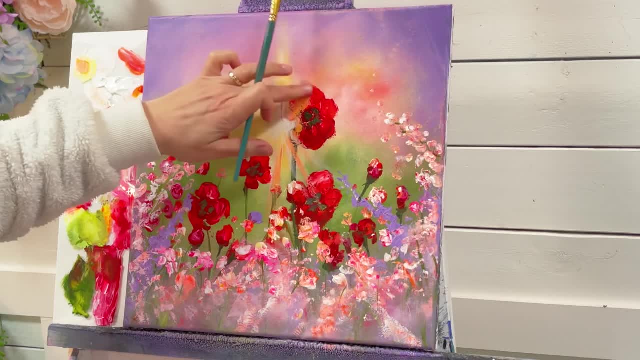 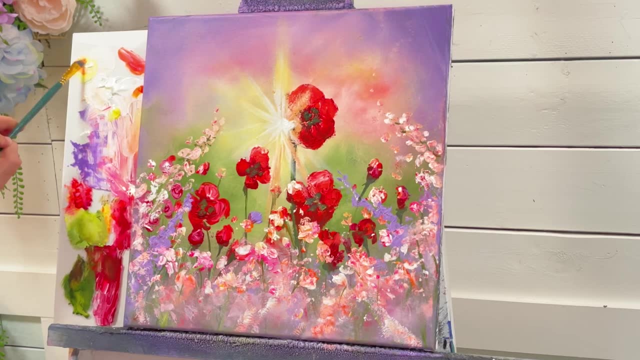 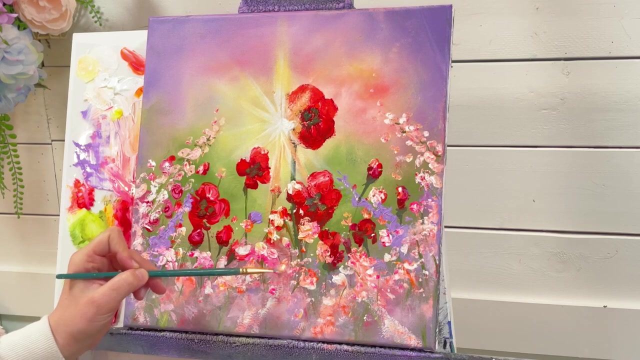 I'm going to mix up the peach again, the yellow and the orange with the white. 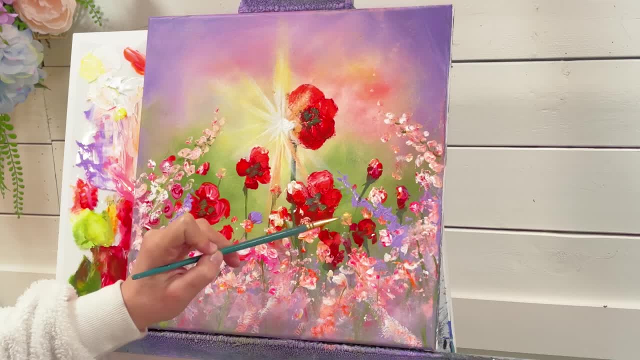 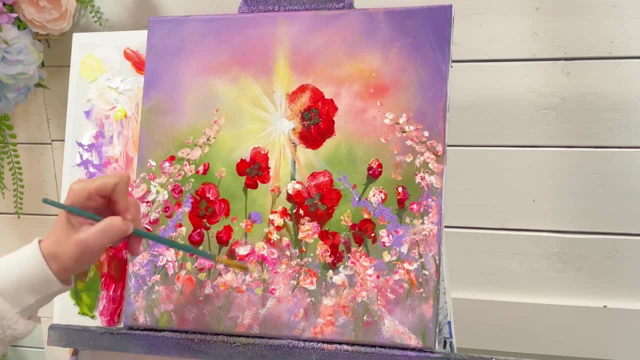 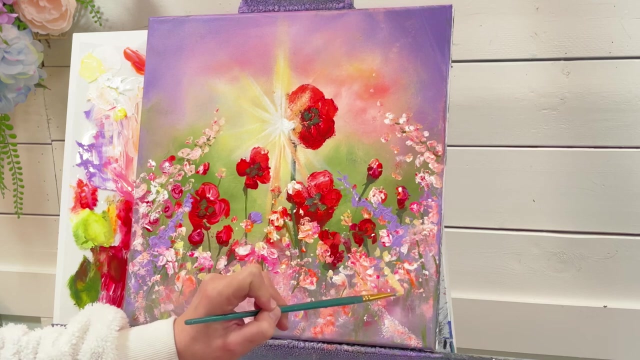 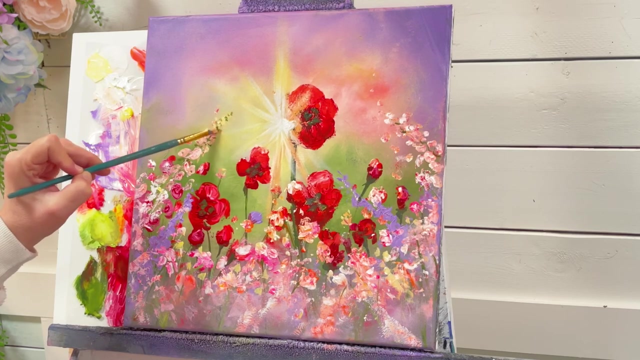 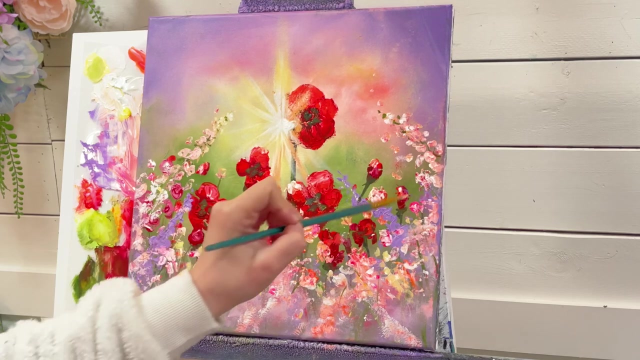 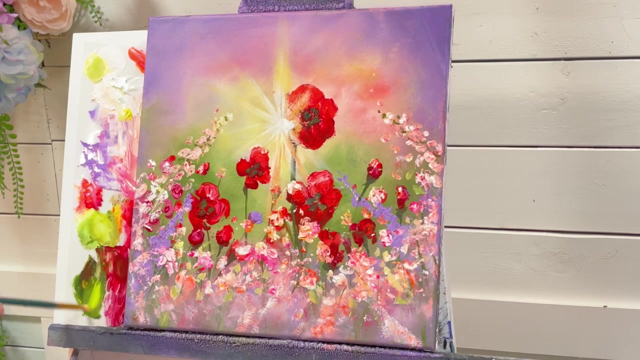 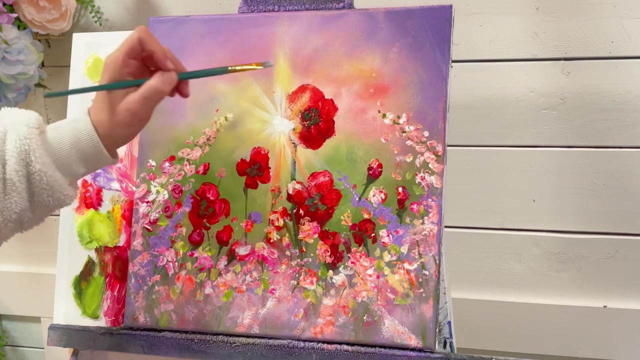 A tiny bit of sap green that I'm just going to get Inside the top of this flower stalk. Mix up a little bit of green, yellow and white, Push and tap for a few leaves. Add the final bit of white in here. 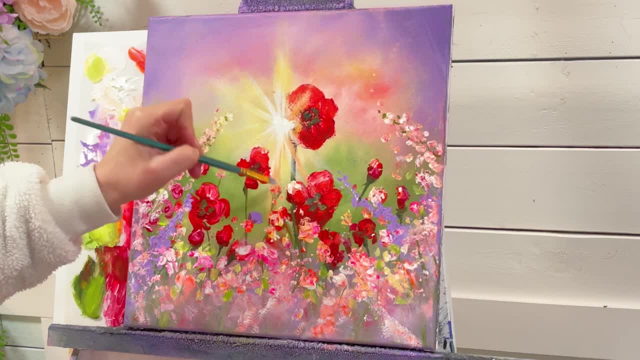 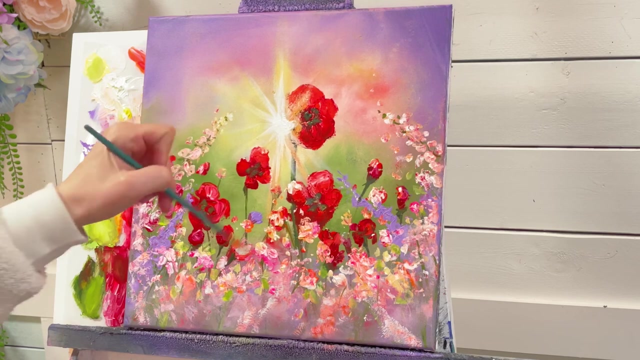 Push and tap on the drop of the flower. A couple drops of red, yellow and white Mix it well. for another few leaves, You can use the base of a pot, Mesh the flower and then add more red in order to make it a little bit darker. 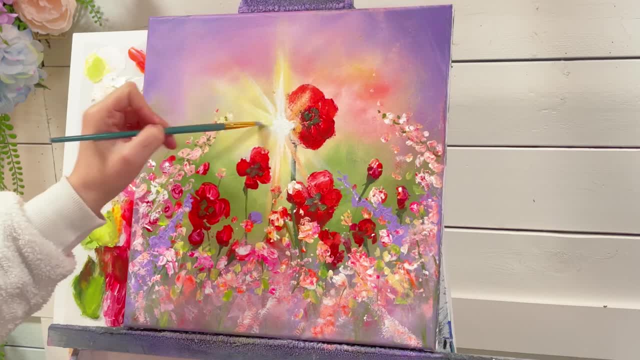 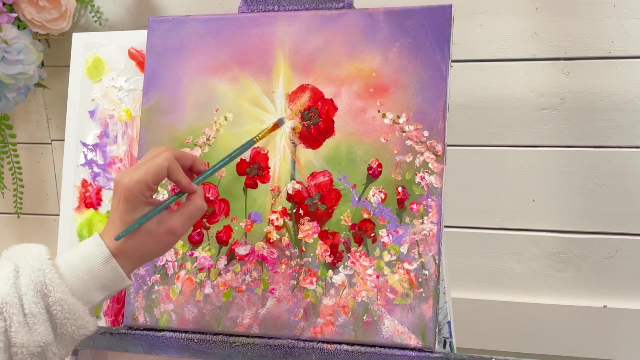 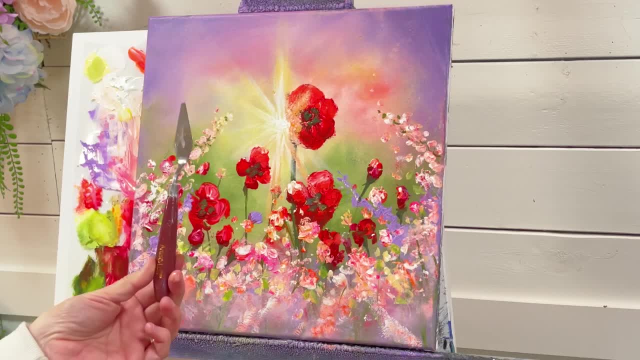 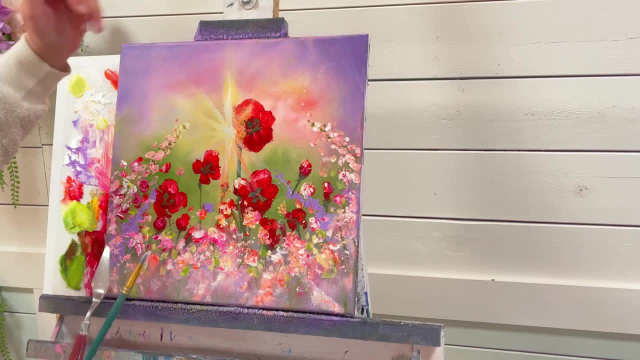 how to paint using some techniques, with a palette knife, a few brushes. Thanks for watching and I'll see you guys very soon in my next video. Bye.